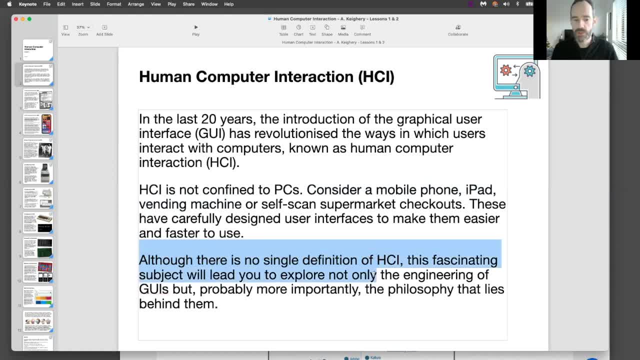 So this fascinating subject will lead you to explore not only the engineering of GUIs- graphical user interfaces- but, more importantly, the philosophy that lies behind them as well. So, yeah, so just try and remember this point about graphical user interfaces, because that'll come up quite a lot. So we call those GUIs And they've evolved, you know, over time. 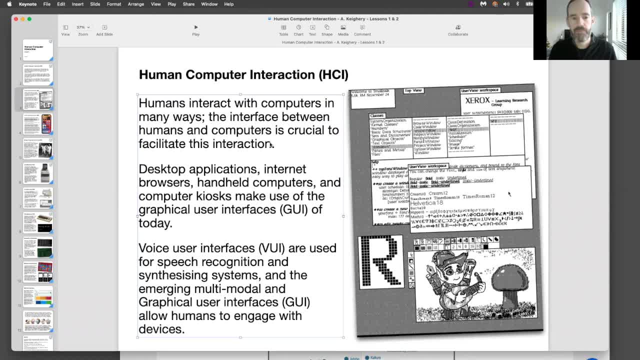 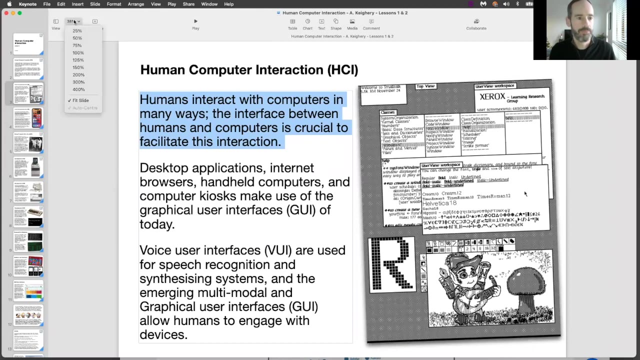 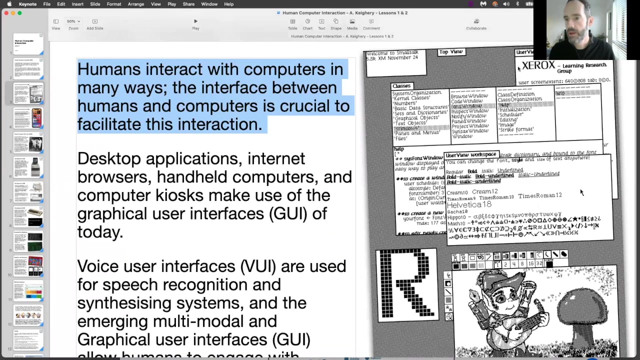 So next slide. So humans and computers interact in many ways, And the interface between the humans and the computers is crucial to facilitate this interaction. So over here on the right-hand side of the screen, let me zoom in a little bit so we can see it. So this is an example of a very earlier interface from Xerox. So like what's, 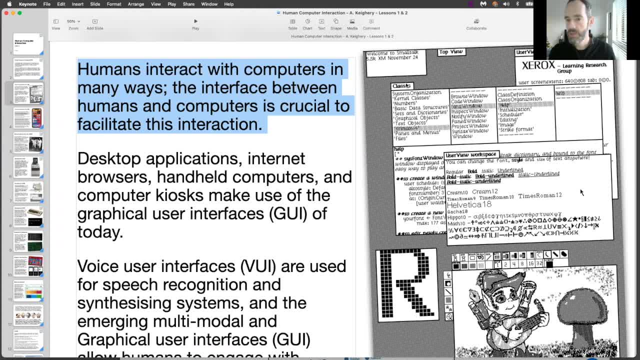 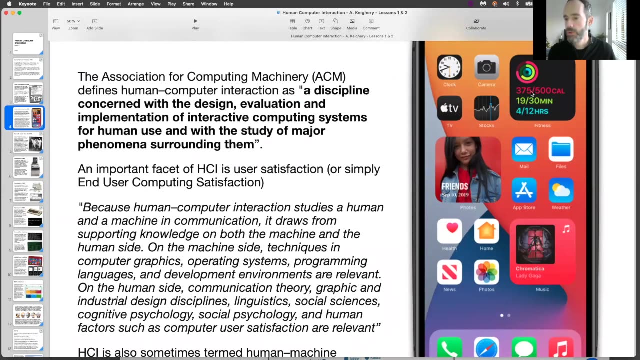 the first thing that would strike you about this interface If you think of the color scheme on it. So what jumps out at you? So say you were to compare this interface with something like this. So this is a modern interface. You all know what this is, don't you? 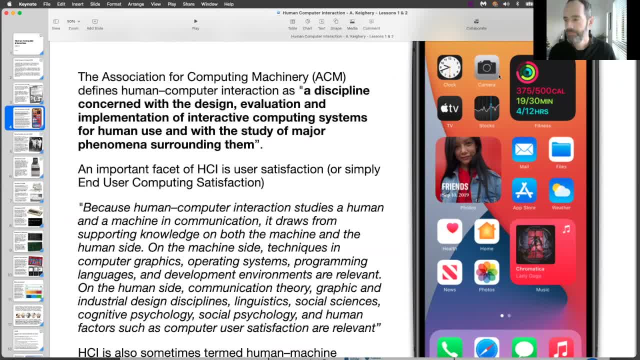 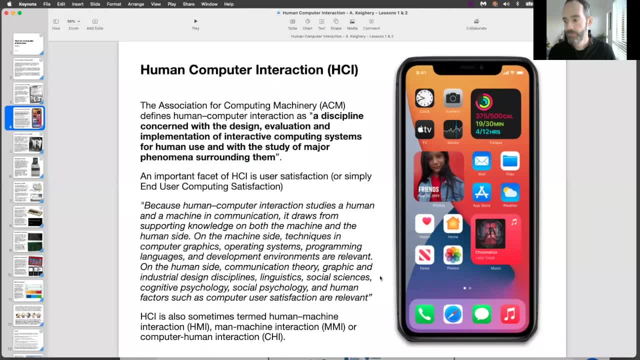 So what's this? the interface from Yeah, so this. so what's this? a representation of Yeah, these are all icons. So the different individual pictures on the screen that you click are icons, right, But in a general sense right. 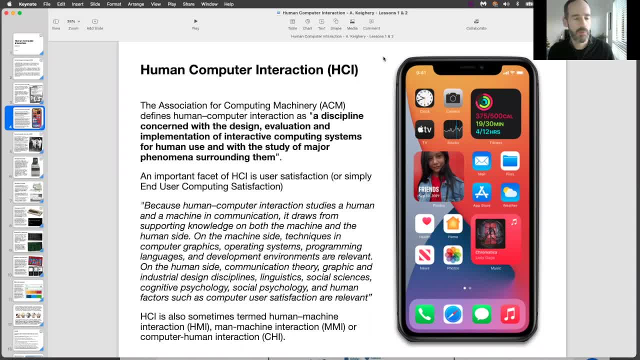 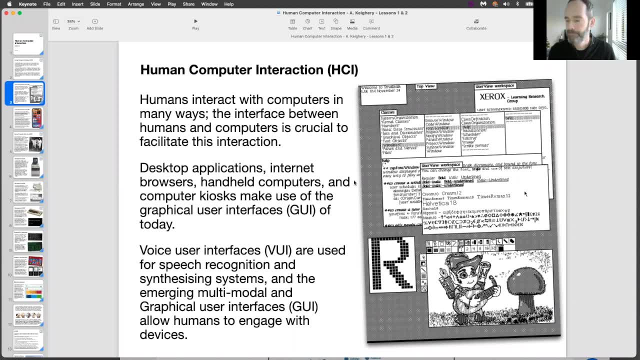 Compare this interface, which is from a modern phone, to this interface. What strikes you as the main difference? So this is an old one. Yeah, the color style very cool. Yeah, so this interface is monochromatic or it's. you know, they didn't have color displays back then. 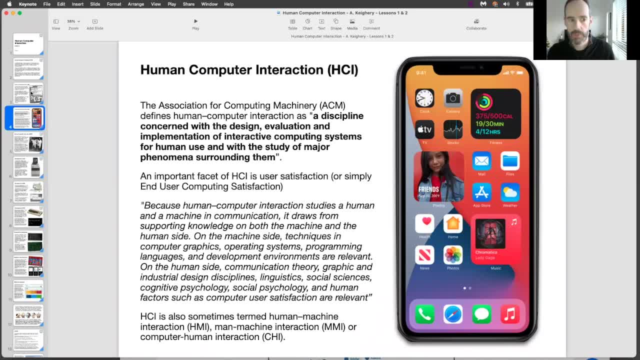 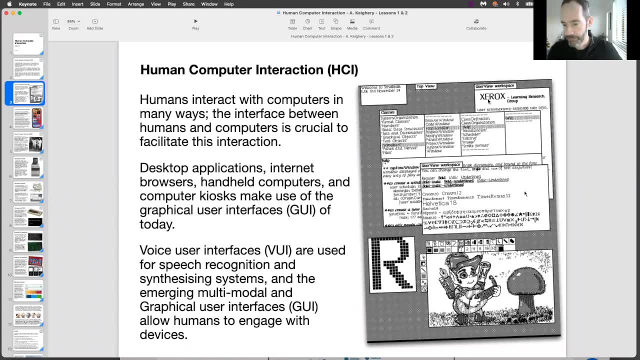 whereas we do now, you know. So this is a an interface from an old Xerox machine, So you were quite limited in terms of the pixels, So the number of dots on the screen. you are quite limited in terms of the 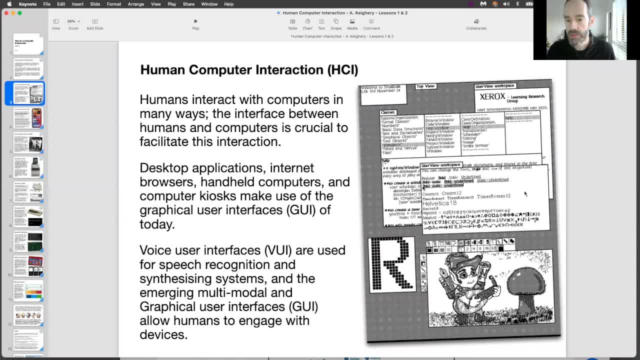 the fonts that it could display, So it could only display certain type of letters and texts, And also the images were limited as well because of the pixels, the dots on the screen And because the screen resolution and also the colors as well, right? So these are all examples of interfaces or GUIs, right? 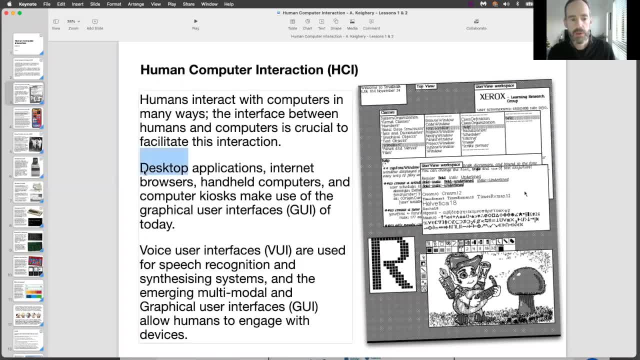 And these allow us to interact with the machines. So desktops, desktop applications, internet browsers, handheld computers, computer kiosks, they all make use of GUIs, right? So that's one way that we can interact with machines. So another way we can interact with machines is by using what they call voice user interfaces, and they're used for speech recognition and synthesizing systems. 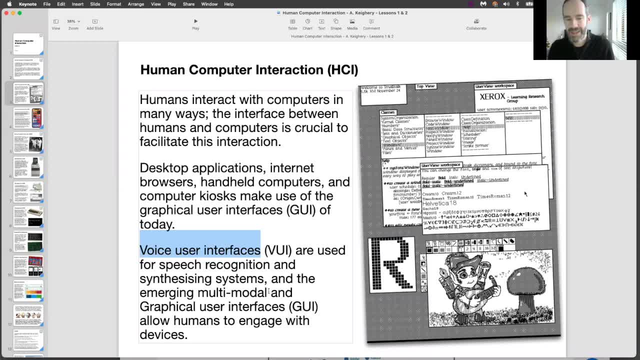 And then you have GUIs or interfaces that are what they call multi modal, So we interact with them in numerous ways and that feedback then can it can be output or we can, we can get feedback from the device right. So could could anyone give me an example of a voice user interface? 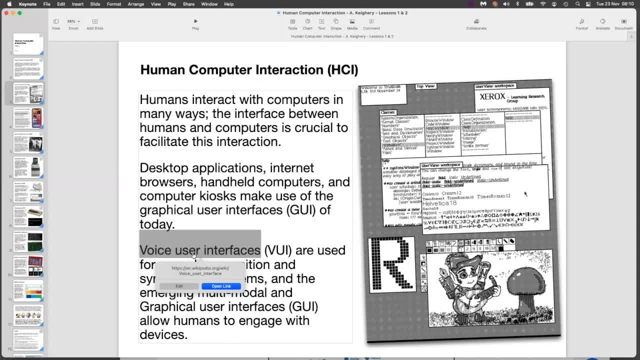 I think, sir, listening to music, Yeah well, listening to listening to music right is, I suppose, when you receive information from the device. Okay, So so how would you give information to the device using your voice? 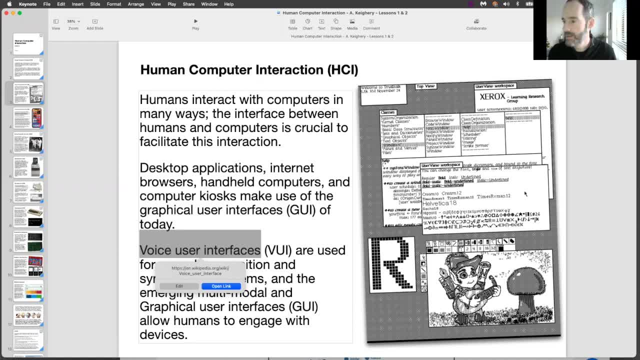 Yeah, okay, And we have a couple of good suggestions in chat right, Google Assistant and Siri. So I can, I can, I can use my, my, my phone here. So I go, Hey, Siri, What time is it? 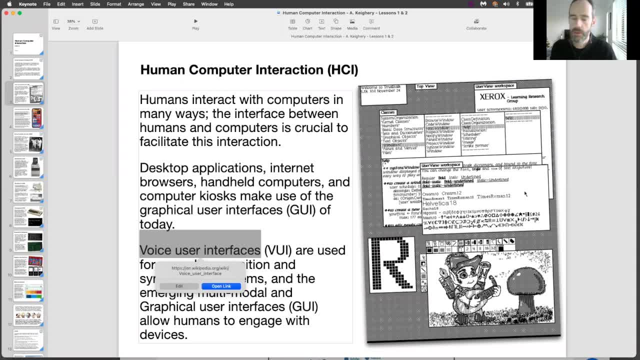 It's 8.10am, Yeah, so you can hear that, guys. So that's an example of a voice user interface, right? And then in the background you have the device converting my voice into a you know something that it can understand, and recognizing my voice as well, and then carrying out the commands of my voice. 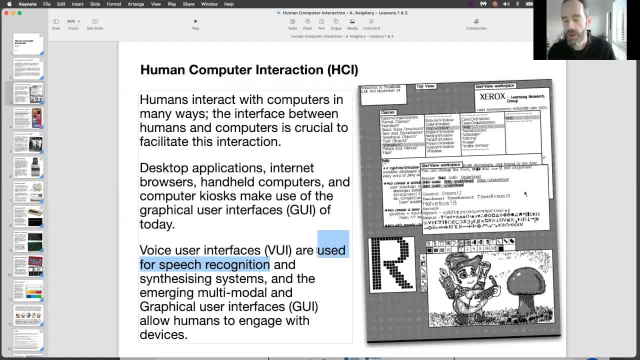 So that's an example of interacting with with a device, Just in a, in a slightly a different way, because when I interact with Siri or with Google Assistant, I don't use my, I don't use a graphical user interface, So I don't even need to be looking at the device to use it, Right? So I suppose just the point I want to make is that there's there's different ways to interact. 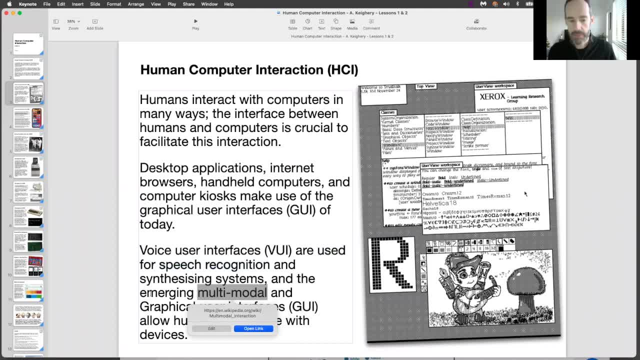 with the devices, right? And what multimodal is right, And now you can. You can see this line where it says emerging multimodal, So that means a device that would give us, I suppose, output, or it can actually take input as well- using multiple sensors, Right, So could it? could anyone give me an example of a multimodal device? Right? So say if you think of something that you might see with gaming. 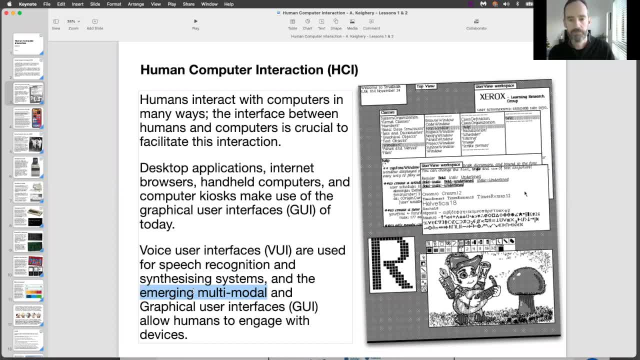 Right, Right, Sorry. does it connect to the different generation of the phones or different like iOS or Android or anything? Not, not really Right. So what I'm thinking about- and let me explain a little bit clearer- is I'm thinking about a device that can send me information right either by sight, or by sound, or by touch. So what I'm thinking about is a device that can send me information right either by sight, or by sound, or by touch. 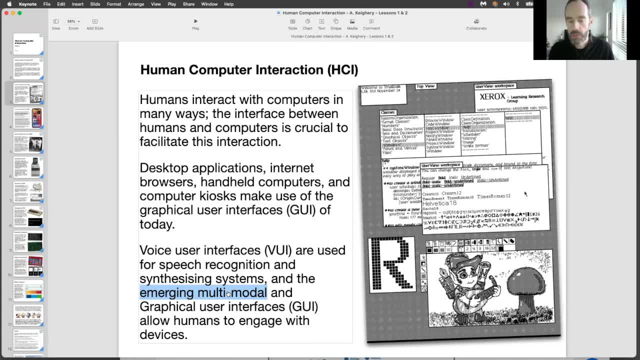 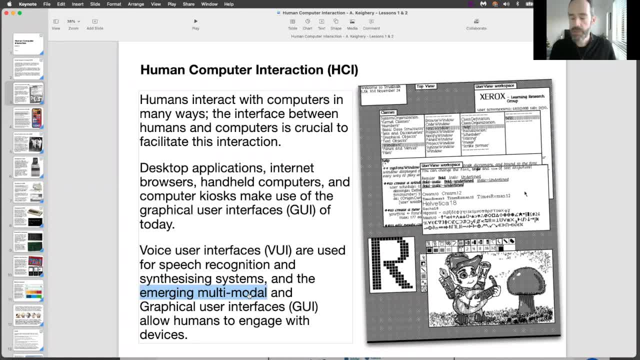 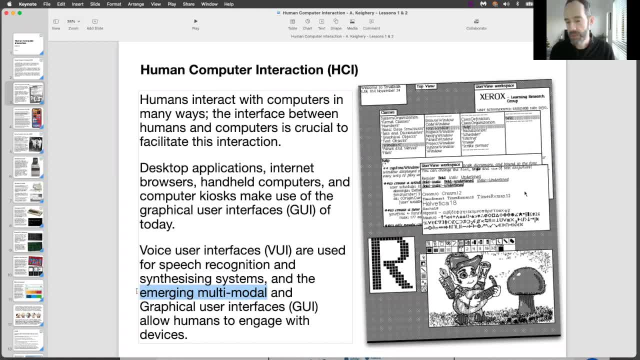 working together, um, as, as best they can, and and look the devices and human computer interaction. it's evolved over a long time, you know. i suppose i just wanted to start off and let you guys know, maybe, where we've um come from and you have these sort of um, these kind of displays. 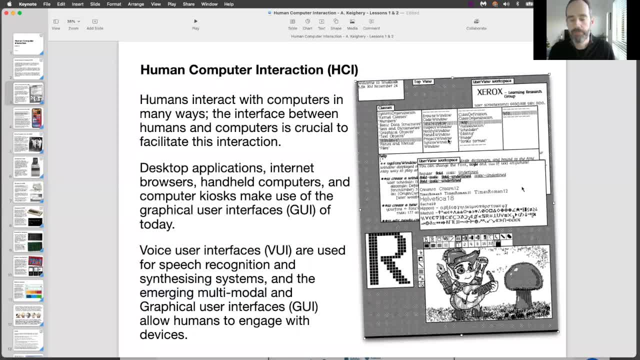 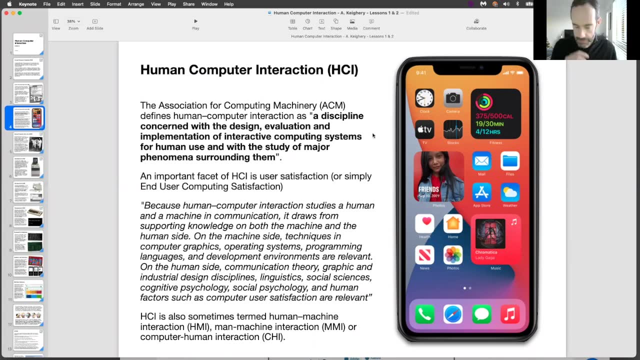 very limited, you know, very um, very gray, not able to render color, um color sort of visuals. and then we've moved on to something like this, which is a lot more, a lot more natural um and look a lot more interesting to look at, a lot more um in engaging. so let's carry on right. let's look at um a 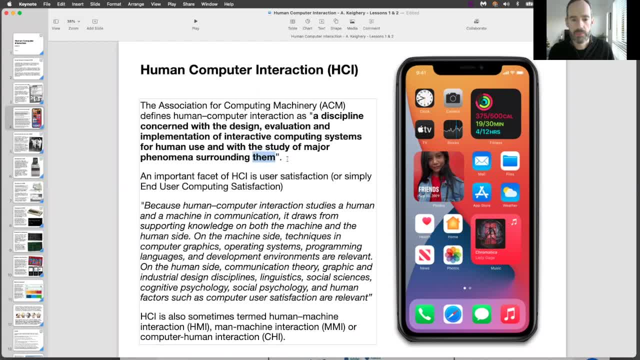 definition right of human computer interaction. right, so it can be defined as a discipline concerned with the design, evaluation and implementation of interactive computer systems for human use and with the study of major phenomena surrounding them. right, so i suppose the important word there is interact. right, because um interfaces need to be interactive. 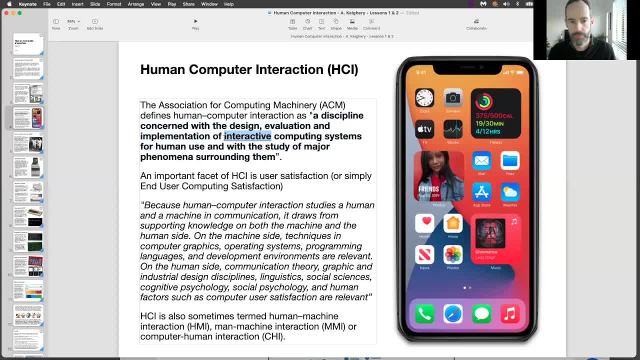 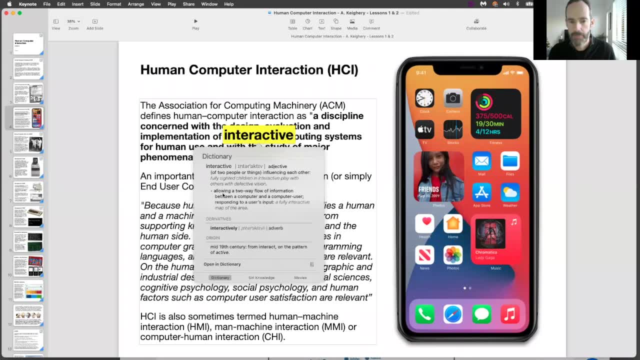 so it's all. what does interactive mean? Look up interactive. So it gives me this definition: allowing a two way flow of information between a computer and a computer user responding to a user's input. Does that make sense? So remember when we're. 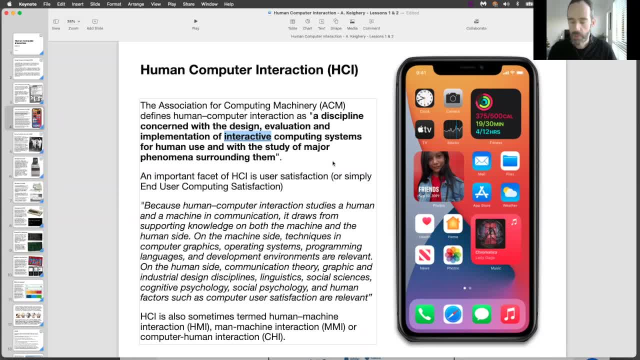 talking about human computer interaction. we're talking about both parties. We're talking about the person, Yeah, And we're talking about the device as well, Yeah. So communicating or linking in, connecting is a good way of putting it All right, So an important facet of HCI. 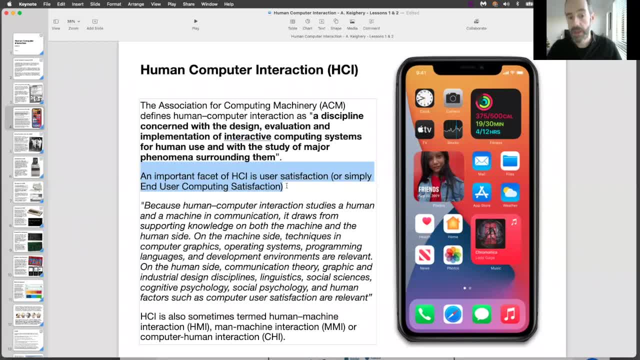 is user satisfaction, Or simply end user computer satisfaction. So what do I mean by that? So, in this sense, what do we mean by satisfaction? So think you're using your phone, Okay, And if you are to continue using your phone, the manufacturers want to make sure that you're. 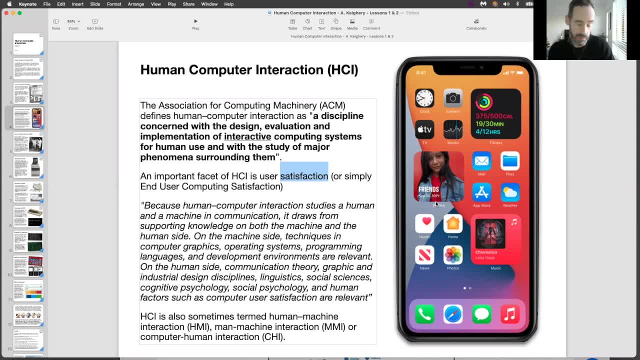 going to enjoy using your phone, And also the app developers. they're going to want to make sure that you're using your phone. So if you're using your phone, you're going to want to make sure that you want to come back and use their app again and again. So this user satisfaction is 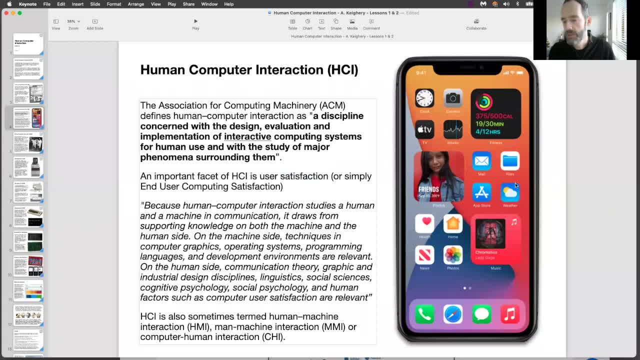 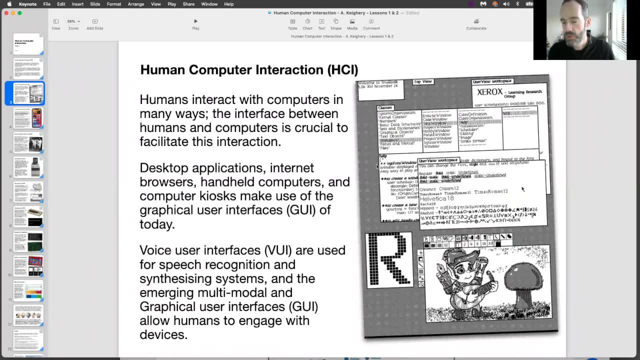 actually really important, Right? So if you were again to compare the two designs, so the new design with the old design, So which do you think is more satisfying, to use Our new design or our old design? Yeah, the new one. 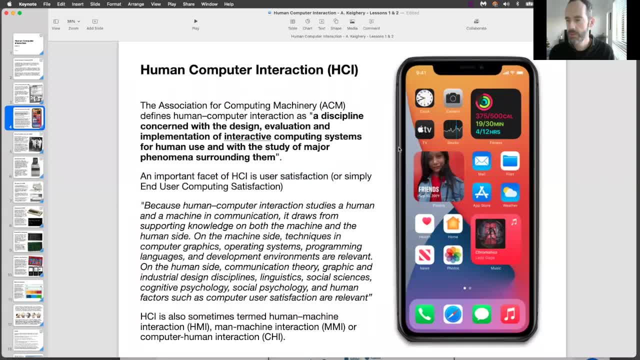 Why, Why, Why would it be more satisfying to use? I think so, The graphic also and also the quality of camera. Exactly, Yeah, Yeah, Yeah, Yeah. Excellent Yeah, Good answer, All Yeah, all the, all the features, all. 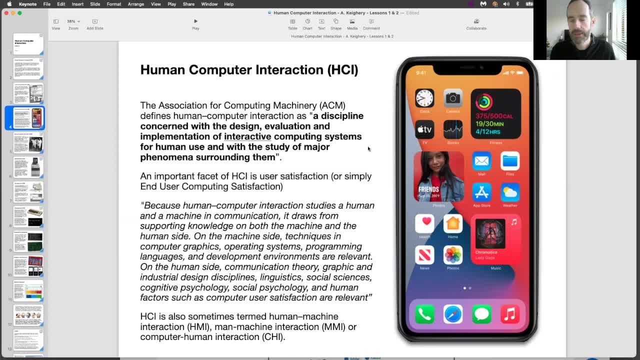 the features on the phone lend itself to being more engaging, more satisfying, More, just just more interesting and but, but but also probably more natural to us as well, you know, because we see in color and most of us do anyway, And and so using a device like this is going to be. 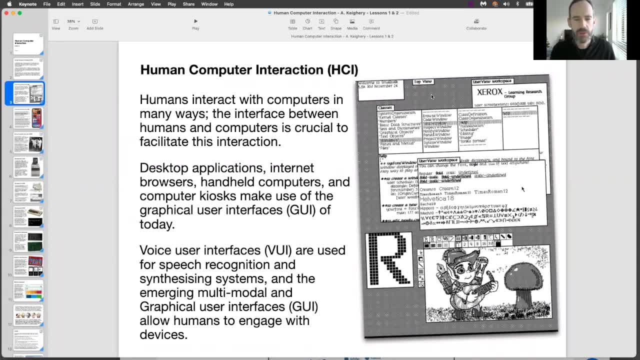 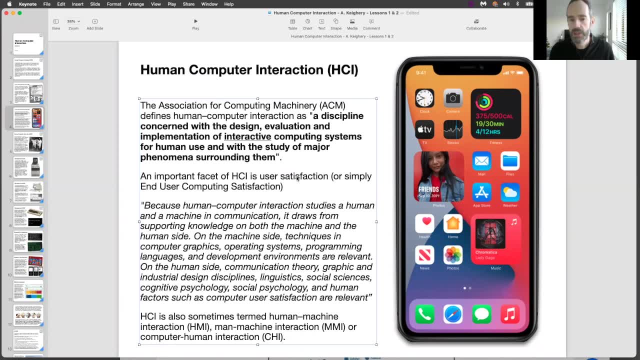 a struggle for us, because we're going to look at it and you know it just doesn't feel right or whatever you know. so this, this user satisfaction, is really important. Right, It's nice. So let me just go through this next section. And because human computer interaction. 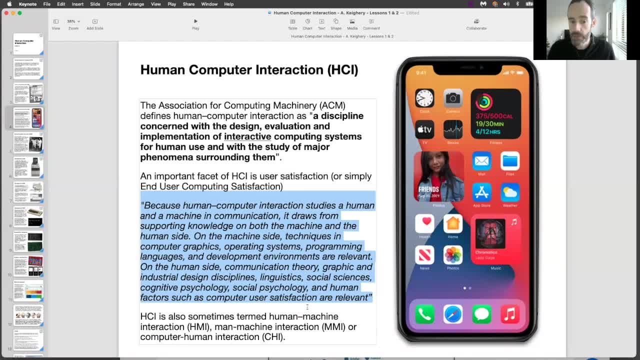 studies a human and a machine in communication. it draws supporting knowledge on both the machine and the human side. So on the machine side, techniques and graphics, operating system programming and development environments are relevant, right. But then on the human size, communication theory, graph and the financial data, the data that's being developed, and then you 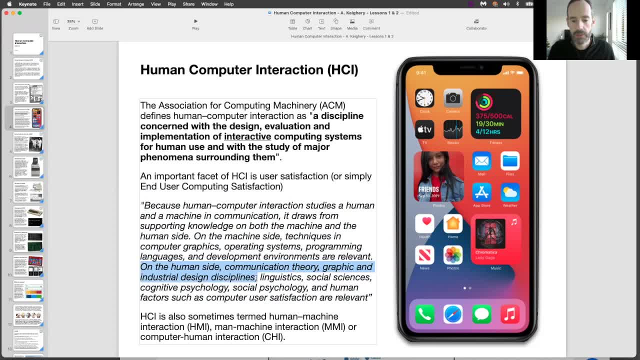 theory, graphic um an industrial design, linguistics, social science, psychology, um, and other human factors such as satisfaction, are relevant, right so so remember you've. you've two um branches to the term human computer interaction, and what we're going to do across this course is we're. 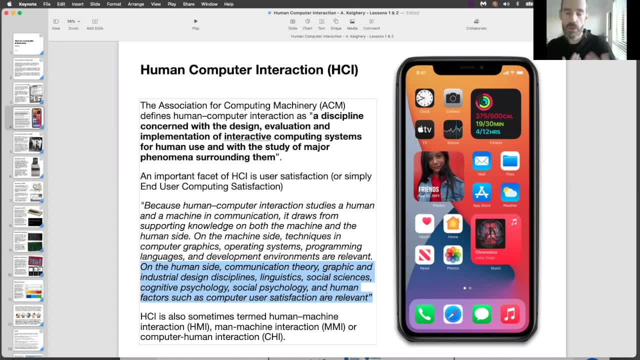 going to try and look at both of those right. we'll try and look at the human side right, maybe some of the um, the psychology behind some of the choices that we make as people, um. and. but we'll also look at the other side, the, the computer side, or the, the the technology um side of things as well. 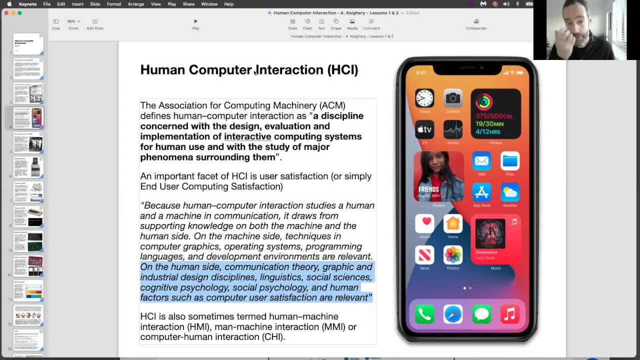 so just, i suppose the point of making is it's, it's a, there's two branches or it's a two-prong definition, right, both. and it has the human element and the the technology element, right um, and that's important, i suppose to to note at this stage. so, so, this course isn't. 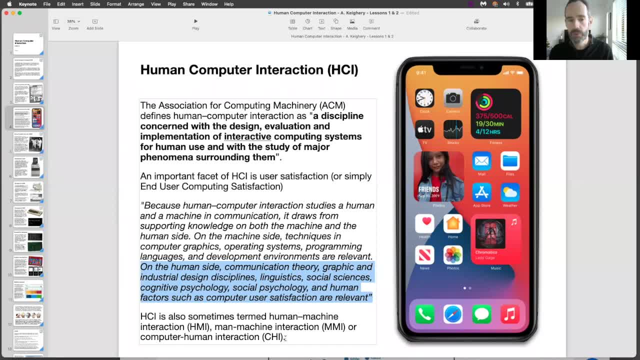 just about um, you know computers. we'll also factor in the the human side as well, um, and then finally, hci is also termed human machine interaction, or man machine interaction, or computer. so so there's other abbreviations, um, for the term, but the most important one is the human machine interaction. 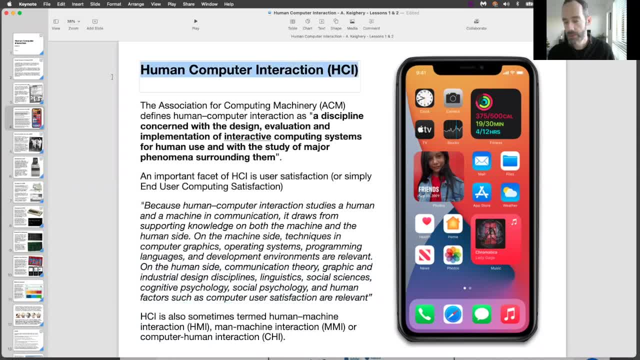 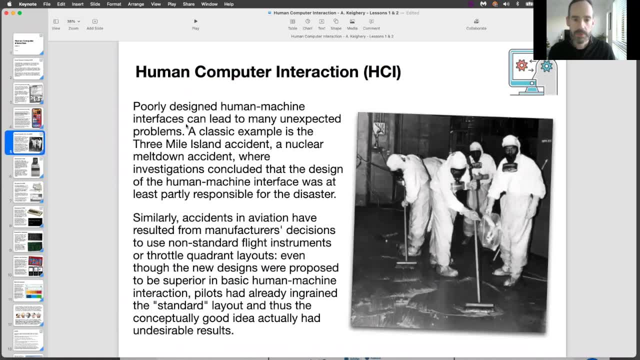 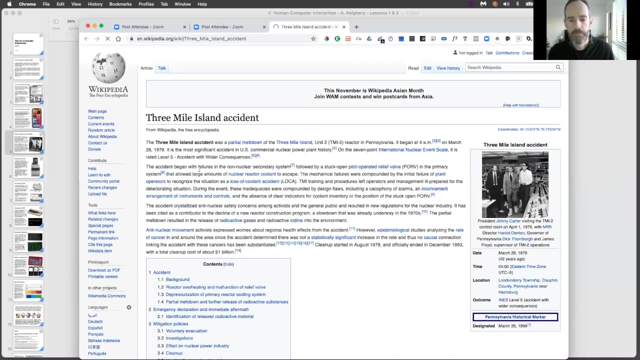 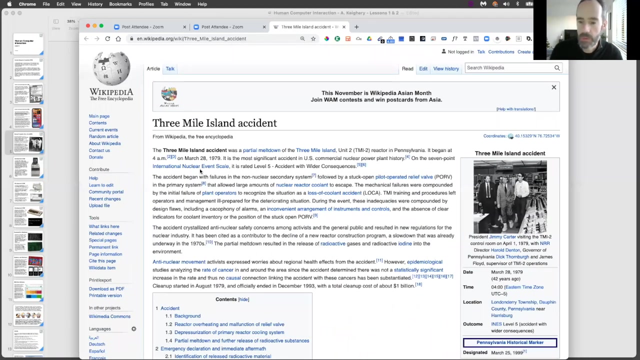 and the most important one is hci: human computer interaction. okay, so that's our little intro um to the course, right? so now this is a picture from three mile islands, right? has anyone heard about three mile islands? can you see that? yeah, so three mile island was what year? 1979, so it was, uh, it was a nuclear accident. so a little bit like 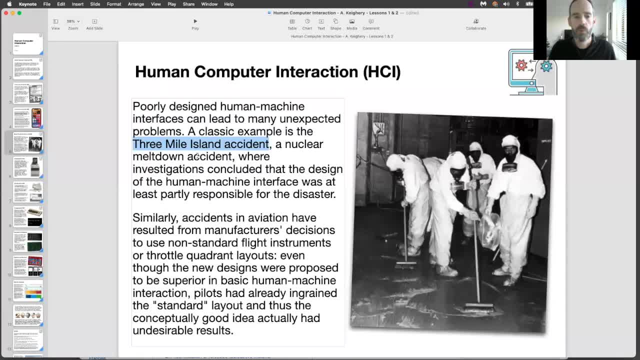 what happened in chernobyl, um, or whatever, and these are the guys that were doing the cleanup after the accident in the nuclear power plant, um, and when they investigated what happened, they concluded that the design of the interface was at least partly responsible for the design of the interface. 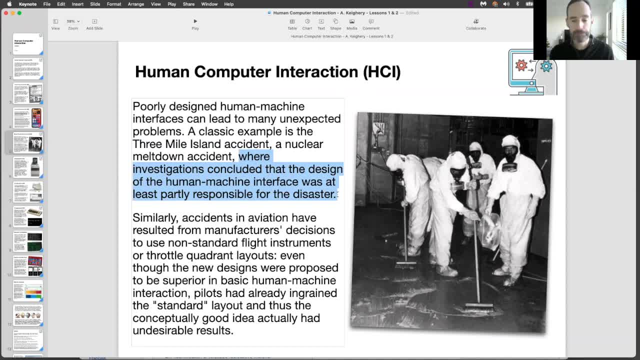 fascinating, so maybe some people can get themselves involved in this because this probably is an Lost Land meat. Each challenging process moving into the new tents you know he was looking forward to saying this call is very exciting and it is an unnecessary, essentially, despite the two- zus. 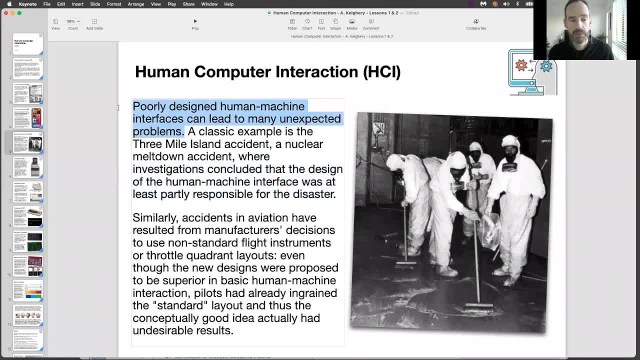 being around for a few weeks. so as a response to the over fiquei left back to się. so you know, some may say: um, let's go backwon though. well, i'm for now. uh, though, it's not like i can trust, hislly can lead to many unexpected problems. So the classic example is the Three Mile Island accident. 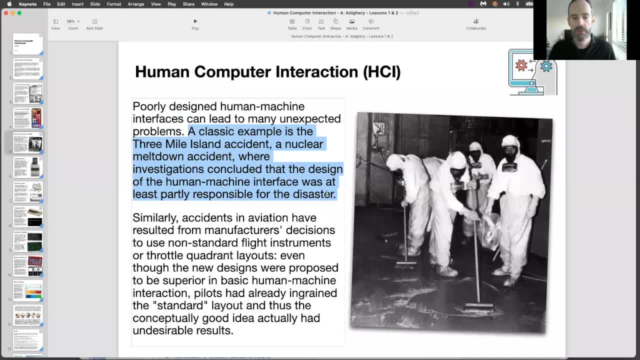 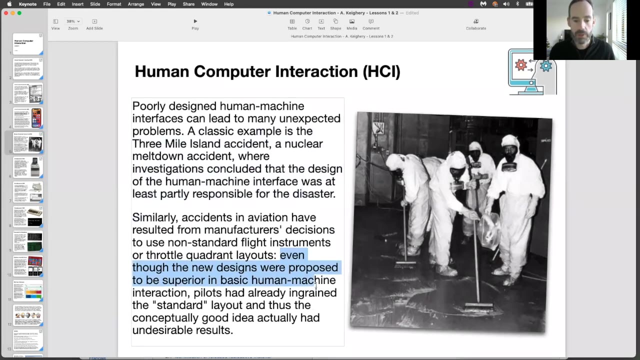 and the interface was at least partly responsible for the disaster. So similar accidents in aviation have resulted from manufacturers decisions to use non-standard flight instruments or throttle quadrant layouts. So even though the new designs were proposed to be superior in basic human-machine interaction, pilots had 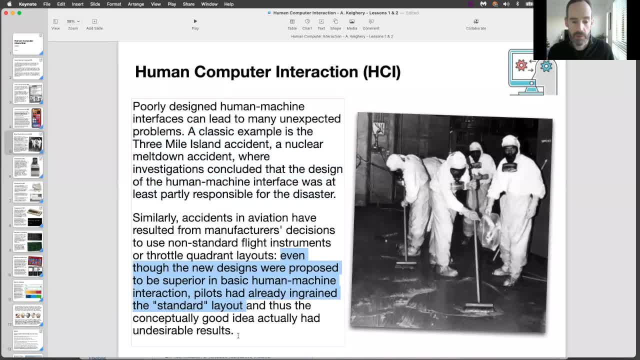 already ingrained the standard layout and thus the conceptually good idea actually had undesirable results. So there's two points we can take away from that. So the poorly designed interfaces or the poorly designed interface in Three Mile Island contributed to the accident, Right? 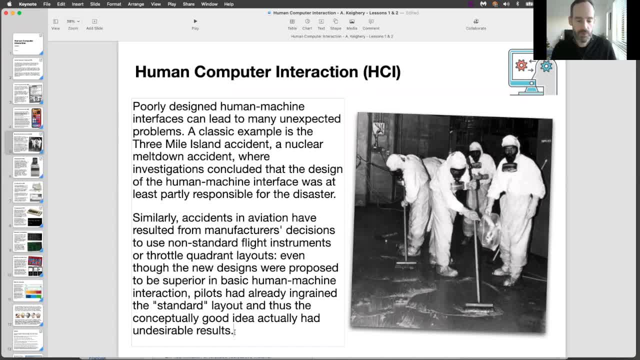 Secondly, in aviation they've tried to change the interface where pilots, you know they change the layout of the switches in the cockpit when the pilots are flying and they've changed, you know, to what they call non-standard flight instruments. Right, 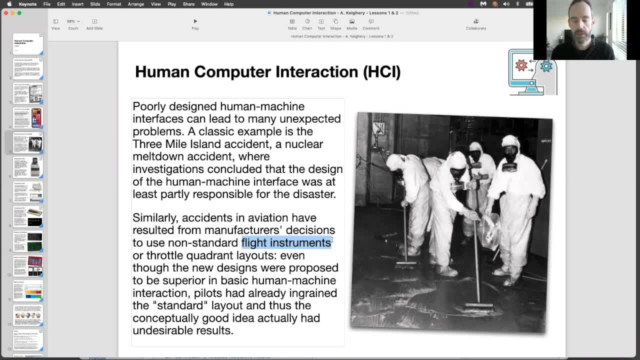 But they've always reverted to the previous design and that they've gone back because they've actually found that the standard interface or the standard layout of the devices was what the pilots were most used to. and you know, learnability is a big factor in interfaces as well, because sometimes you expect: 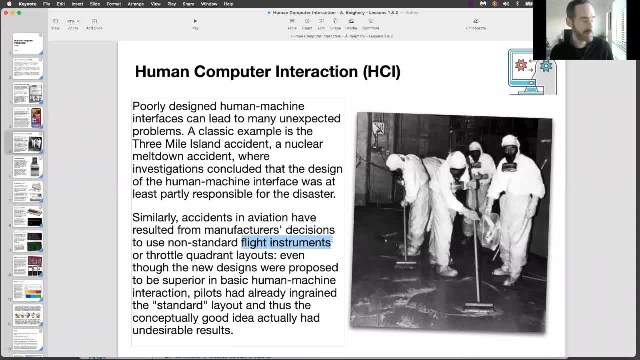 things to be in certain locations and from previous experience, and one of the ways you can measure interfaces is in terms of their learnability. So the pilots had all expected the layouts to be in a certain way and what was a very good idea in paper, you had a designer or a 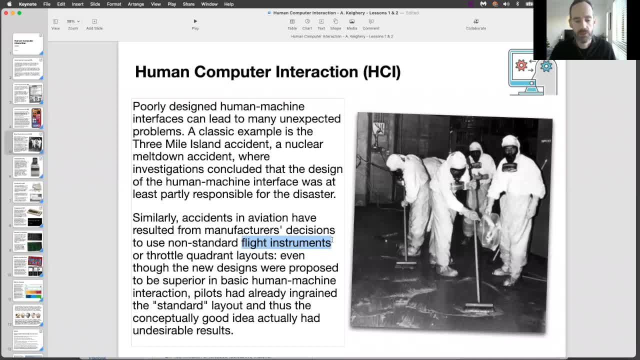 HCI expert sitting down and trying to redesign the layout. it just didn't work in reality, So, and then they always reverted back to their previous designs. So two points to take away. Number one that user interface design is very important And you know it can cause accidents if it isn't done properly and tested properly. 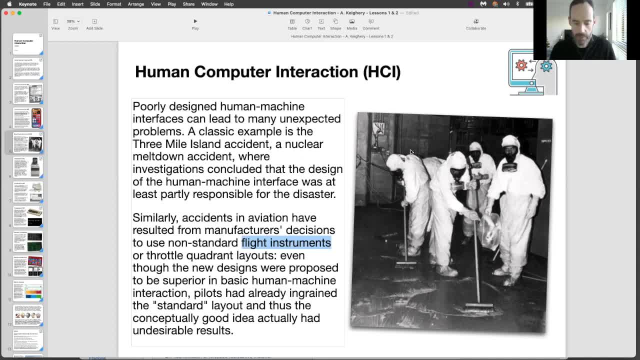 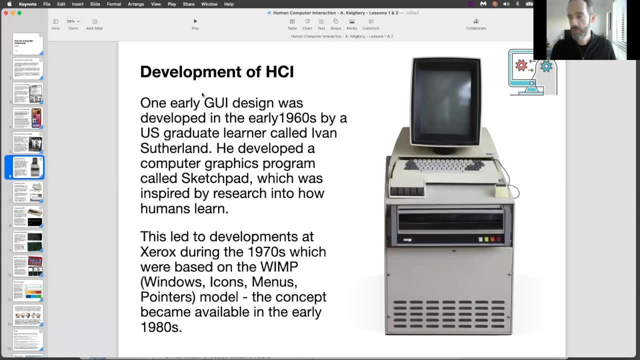 but then also factor in learnability on systems as well. Okay, so we'll just go through- So that's just a little bit of background on general HCI, what it means, the different types of branches to the definition. and now what we'll do is we'll go through the development of human computer interaction. 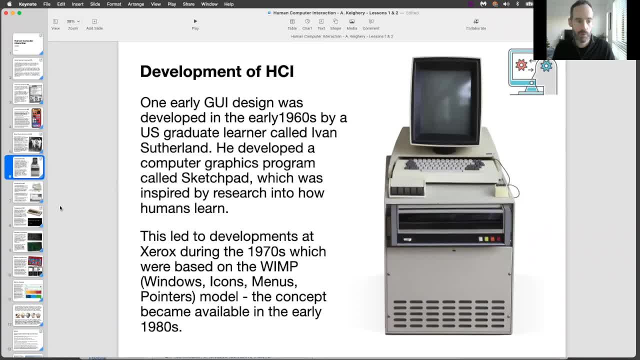 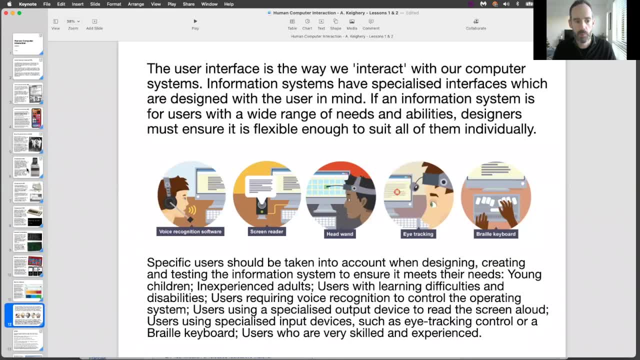 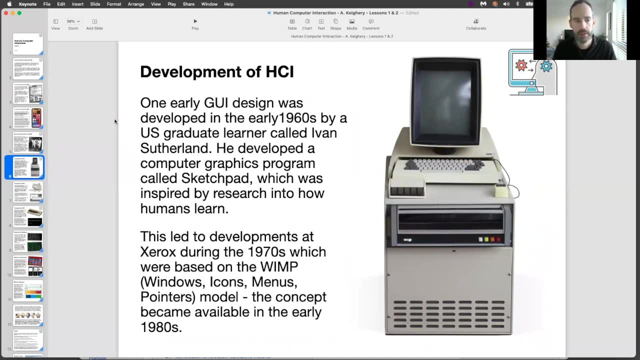 And we'll go right back to the 1960s, We'll go through the different evolutions of design and we'll bring it right up to today. So we'll do this. we'll go through the history for about 10 minutes And please stop me. if you've any questions, just ask a question or you can. 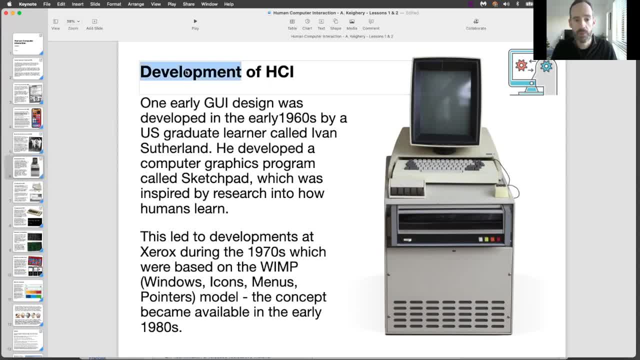 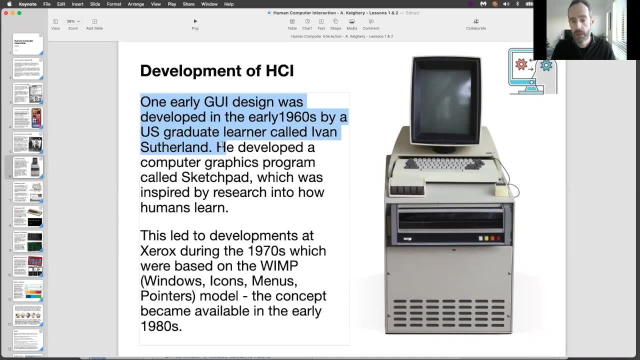 post your question. So the development of HCI, so how we've got to where we have today. So one early GUI design was developed in the early 1960s by a graduate called Ivan Sutherland, And he developed a computer graphics program called Sketchpad. 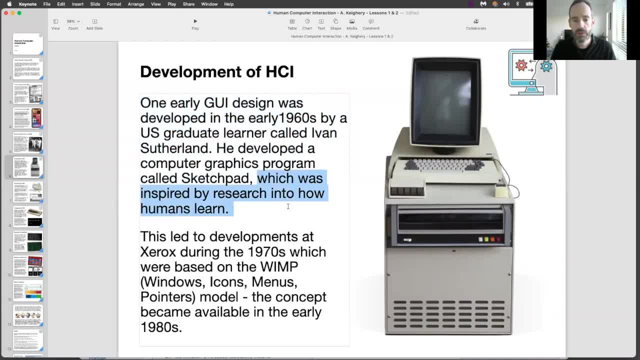 which was inspired by research into how humans learn. So this led to developments at Xerox during the 70s which were based on the WIMP system. So WIMP stands for windows, icons, menus, pointers, And this concept became available in the early 1980s. So we still use this concept today in 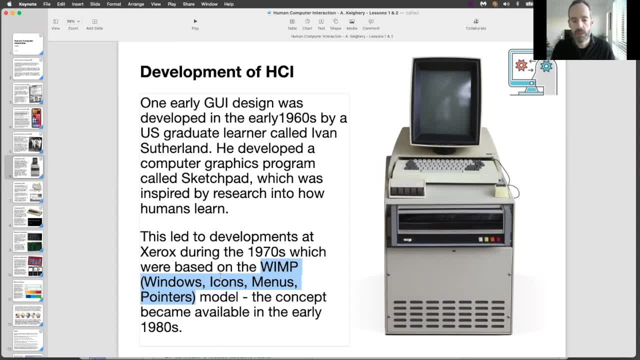 modern computing We have windows icons, menus and pointers. So my pointer is my mouse or my mouse cursor. So if you look kind of close up you can see that I'm going to be using a mouse cursor. carefully at the picture, zoom in a little bit. you can actually see a very rudimentary 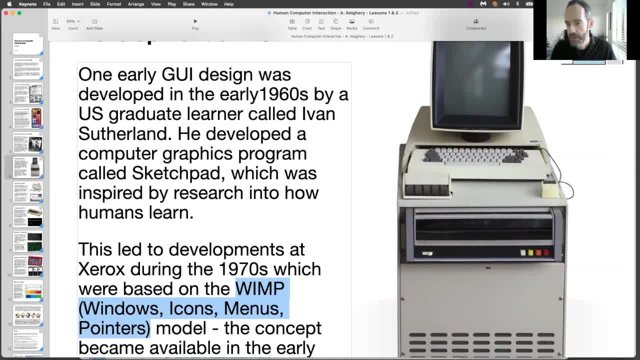 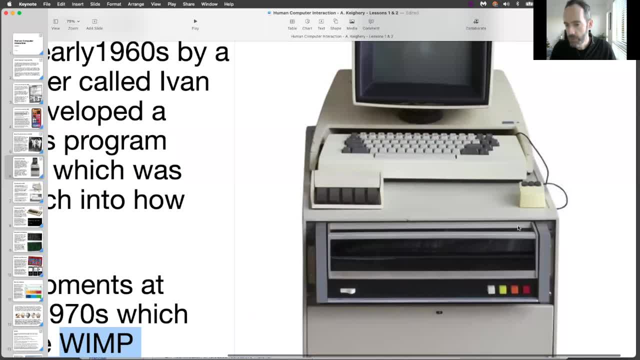 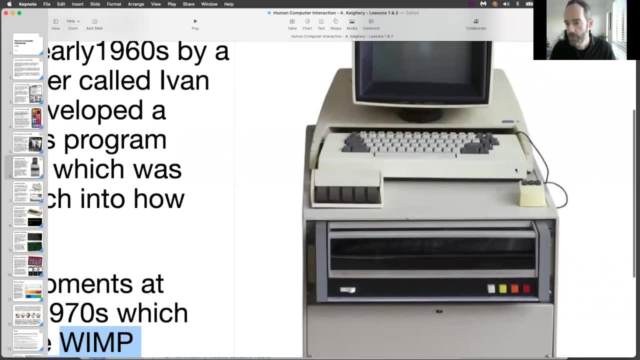 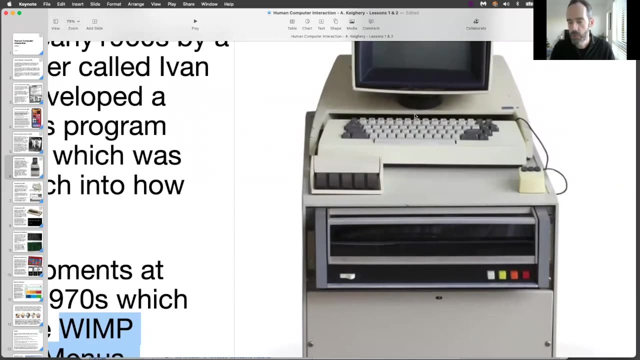 sort of mouse and keyboard. So it doesn't look totally dissimilar or different from what I actually might have on my desk here in front of me with my desktop computer or my laptop. So you have the same components: you have a mouse, you have a keyboard, you have a screen. 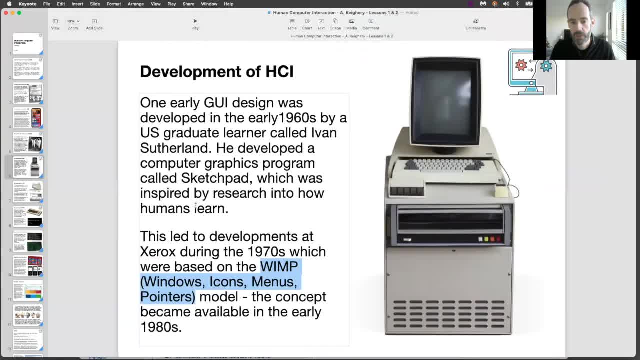 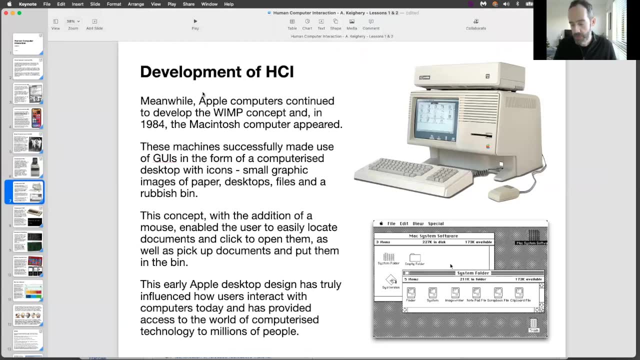 that sort of that sort of thing, Right? So this started back in the 60s and then developed in the 70s into this WIMP system that we still use: Windows Icons, Menus Pointers, Okay, so then I suppose that design was popularised in the 1980s by Apple Mac. 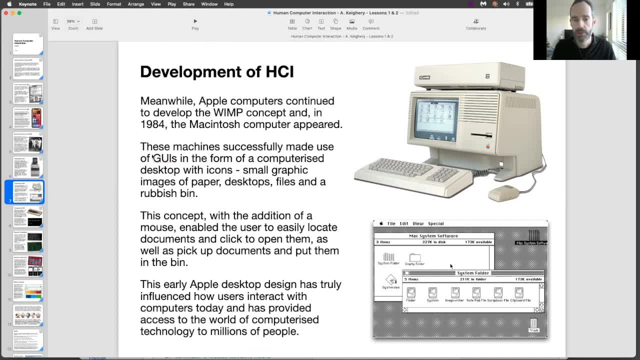 and the Mac Macintosh computer appeared. These machines successfully made use of GUIs in the form of a computerized desktop with icons, And icons are small graphic images, papers, desktop files, rubbish bin these sorts of these concepts. these were popularized in the mid-80s. 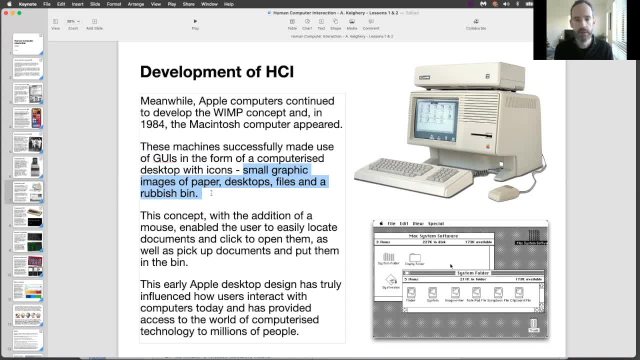 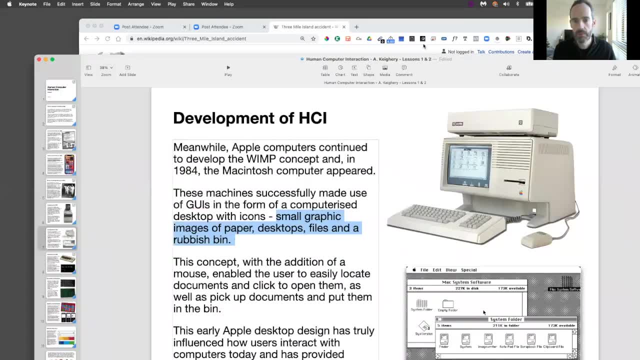 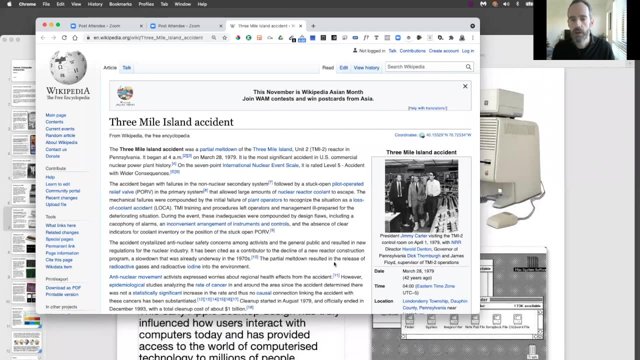 by Apple And we use a very. we use a very similar system today, where we have, you know, windows that we can move around the screen. right, We have layers in the windows, So you'll notice that the window that I'm working on right now is the one that is closest to me. 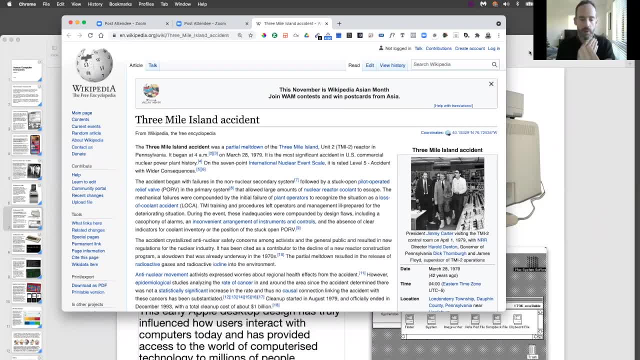 So we have this concept of layers, where whatever I'm working on now is in the front And whatever I've been working on is in the front. So whatever I've been working on now is in the front And whatever I've been working 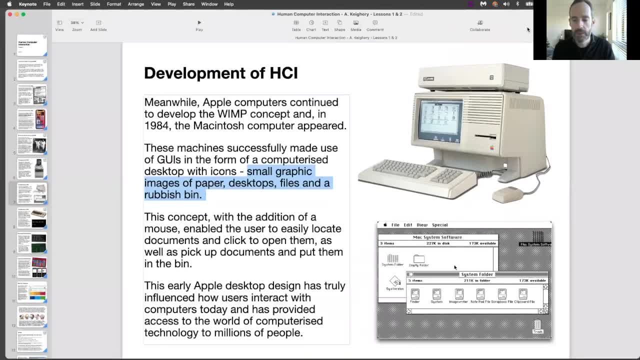 in the back and you can switch between um layers. you have these icons, like the trash icon, and when you pop something in the trash it might make the sound of a piece of trash, and and all these sort of um concepts to try and make things more, uh, lifelike, um, and this concept with the addition. 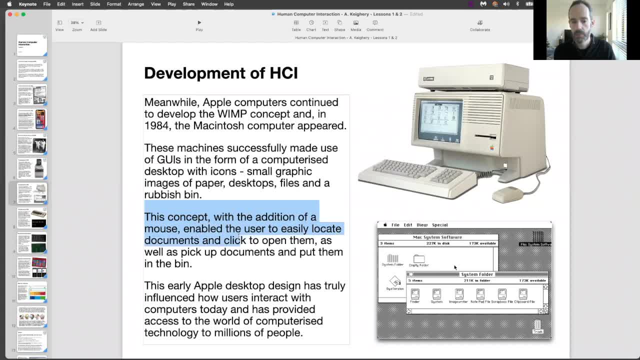 of a mouse enabled the user to easily locate documents and click to open them, as well as pick up documents um and put them in the bin. so if I had a file, I can grab the file, I can physically pick it up, or if I click on this icon here, I click and I hold and then I can move the icon around. 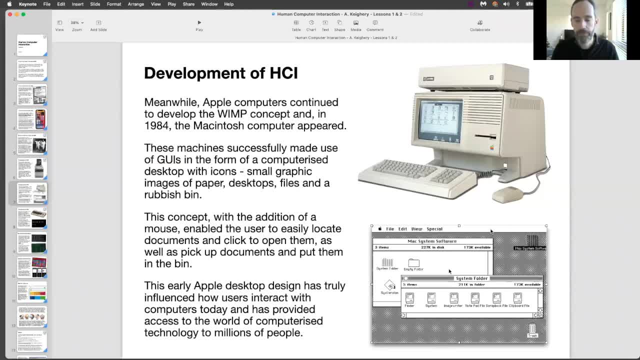 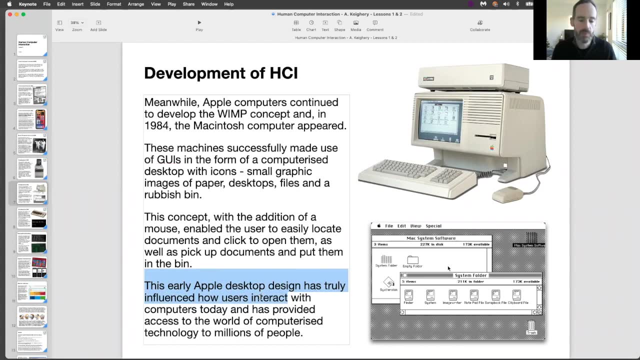 so these are quite revolutionary um concepts at the time and they really um you. you changed how people interacted with with machines. so so this early apple desktop computer design truly revolutionized and influenced how users interact with computers today, and it's provided access to the world of computerized technology to millions of people. and then, of course, apple did. 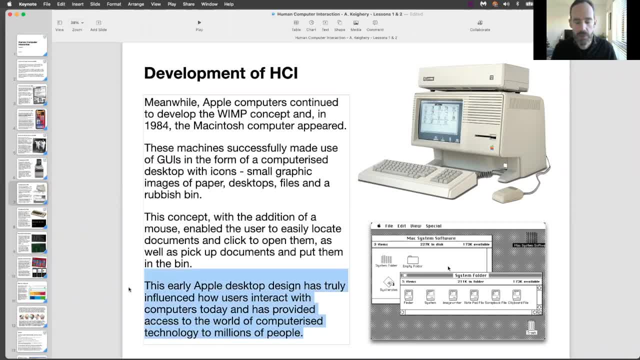 exactly the same thing again, um, some years later. so what? what was the second device that they came up with with that had quite a revolutionary system? there's been maybe three. so if you, if you think of this, this um computer device, as the original device, what was the next device? they? 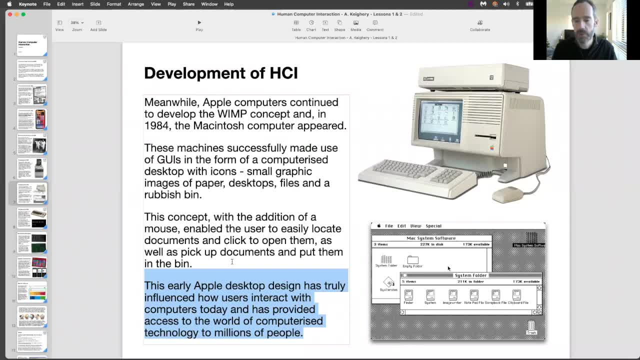 they redesigned and it fundamentally changed how people used and and consumed. so what was the next big device for apple after this? does anyone know? i think, sir, iphone 14, i it could. okay, maybe before the iphone. so so what came before the iphone? uh, iphone 13 plus, yeah, yeah, so even before the phones. so does anyone remember these? 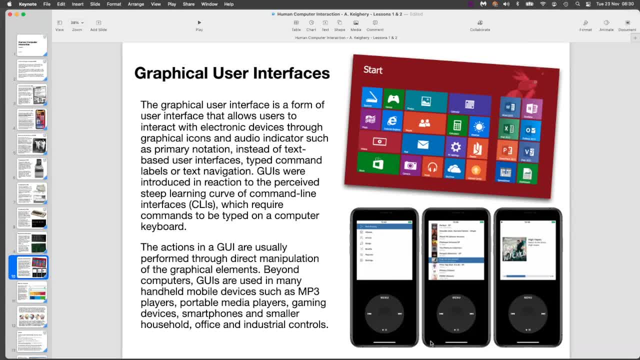 ipad, an ipod, yeah, yeah, so it was the way. um, it was just a new way at the time for people to consume music. um, and again, it was quite clever in that, in that you had a very simple way to interact with the device, so you just had a sort of scroll wheel down here and that moved. 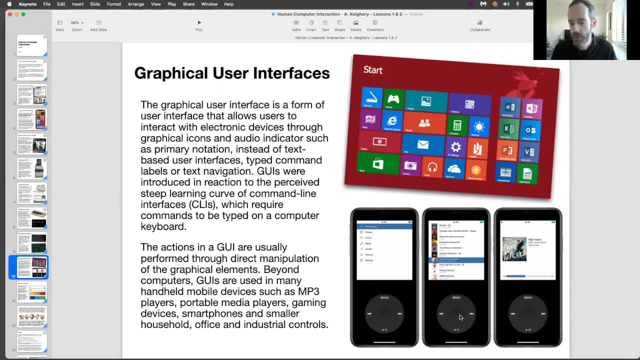 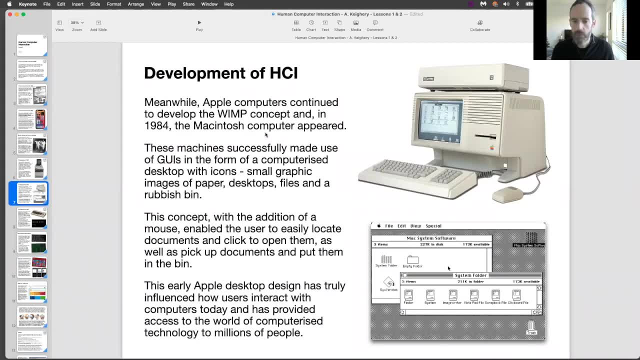 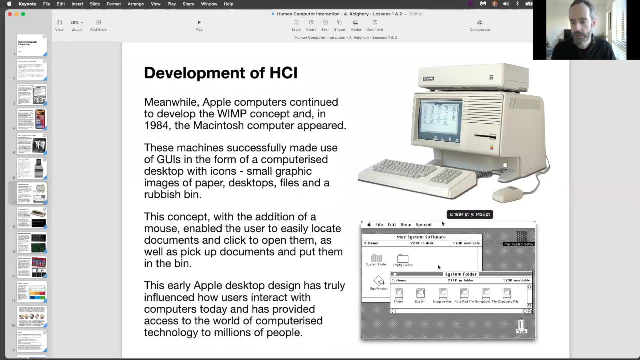 up and down and then when you got to the song you wanted, you pressed click. so so apple have done this in, in terms of design, um three or four times, you know, going right back to um 1984, and this concept of windows and pointers and icons and all that but wimp stuff we spoke about. 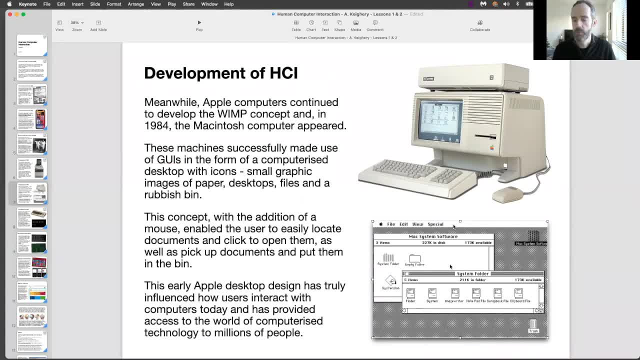 and then they've done it again, um, in terms of the, the ipod, and, and you know, fundamentally that changed how people consumed music. um, and they've, you know they've done it more recently, like an example you gave with with their um, their iphone designs, right. so again, um apple. 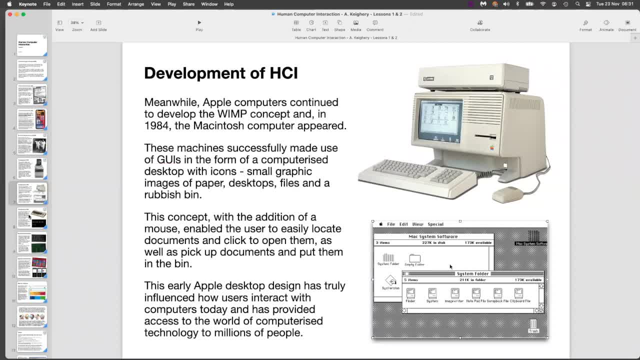 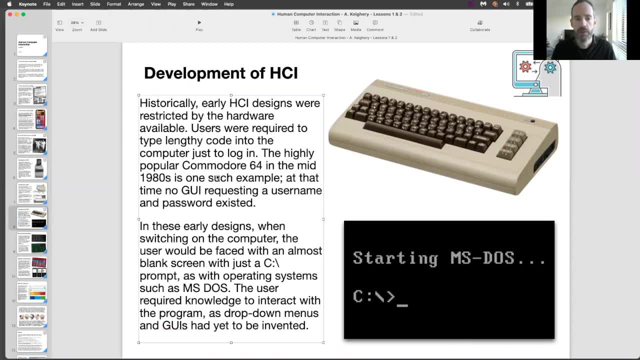 um, and then they've done it again. um, in terms of the, the ipod and, and you know, fundamentally would be a big part of the the story of interface design. okay, so we'll, we'll move on right. so, historically early hci designs were restricted by the hardware available and users were required to type in. 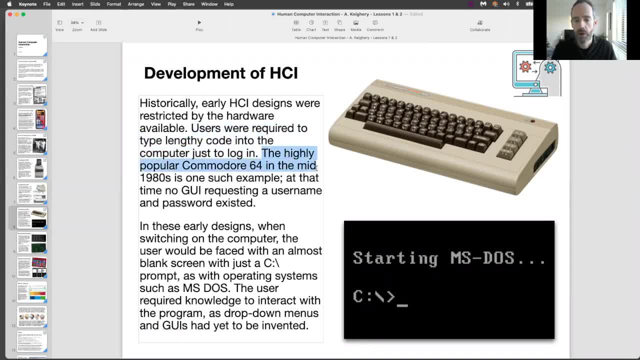 lengthy code just to log in. so the highly popular commodore 64, which is this, is one such example. um, and at the time no gui requesting a username or password existed. so my cousin actually used to have one of those computers and you would turn the computer on and it didn't do anything. you you had. 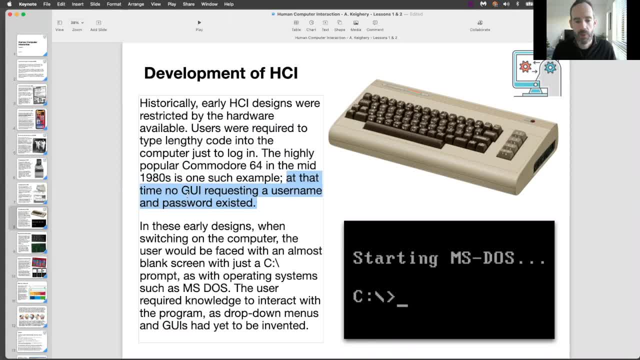 to you know know how to do even the most um basic task? because it was this, it was this um command line prompt right, and, and that meant the. the computer responded to text in the computer and it was a text input. so you needed to type in the commands and then you'd hit return and then the. 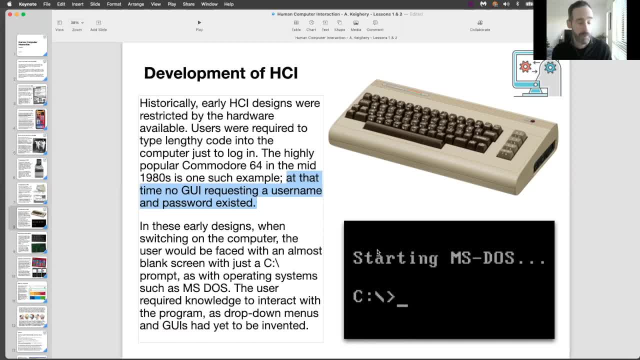 computer would carry out the command that you typed in. but if you made any mistakes, or if you- if you're you know- you didn't know the commands or your typing was incorrect, then the computer wouldn't be able to do anything. so those early designs: when switching on the computer, the user, 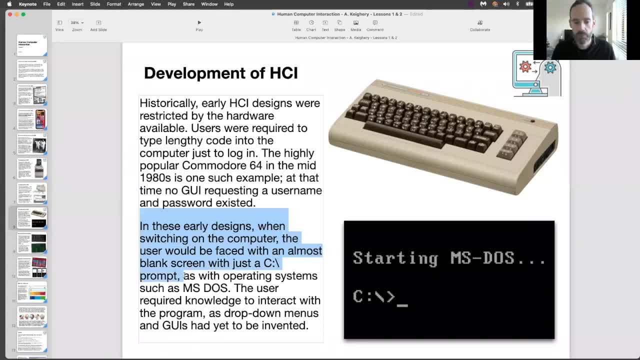 would be faced with a blank screen with just a c prompt. um as we're operating systems such as ms-dos and the user required knowledge to interact with the program. um as drop down menus and guis had yet to be invented, so so this. so this was right. um. 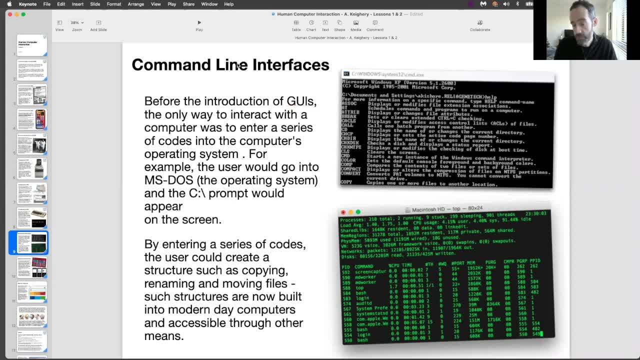 before that um. so an another device or another way of interacting with with the machines is through what they call a command line interface. so this is different from um, a GUI system, where you've got icons and Windows and a pointer and a mouse and this sort of stuff. 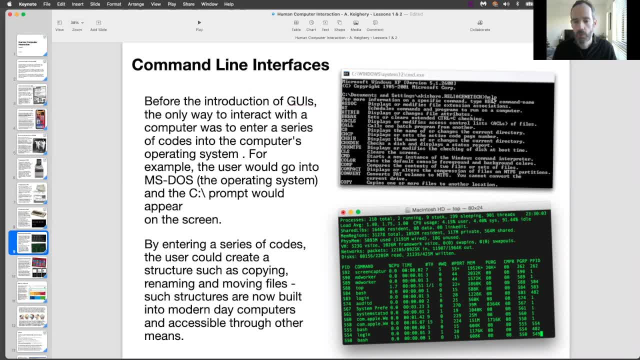 so this is text based commands where you actually type in. so on the top you have um- this is the command prompt on Windows, and then the bottom here, this is the terminal um window on Mac OS, and what it does is it asks you to type in your instruction. 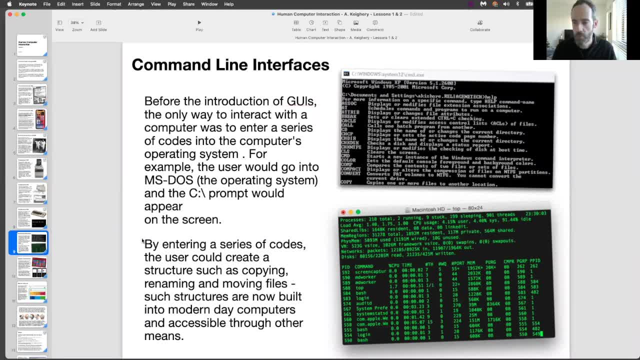 um, you hit return and then you get information back from the computer in the form of text, so very difficult to use and very specialized to use is as well, because you, you, you, not only need to know the language to type in, you also have to interpret the results back, so you get back a whole. 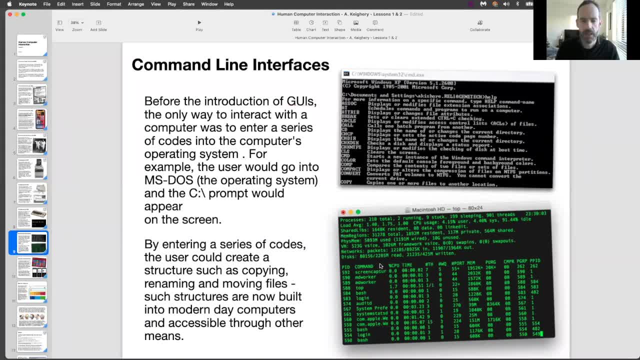 load of stuff like this and you have to try and understand it. so it can be, it can be difficult, but again, another way to interact with the device. it's called a command line interface, right? so before the introduction of GUIs, the only way to interact with computers was to enter a series of codes into the computer's. 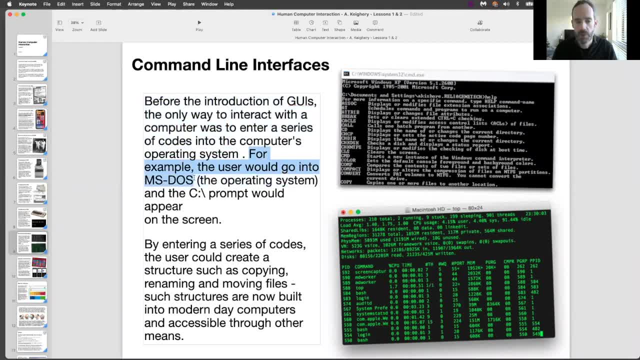 operating system. for example, the user would go into MS-DAS and the C prompt would appear on the screen, and by entering a series of codes, the user could create a structure such as copying, renaming and moving files. and such structures and methods are now built into modern day computers, but they're accessible through other means. so so how would we you know? 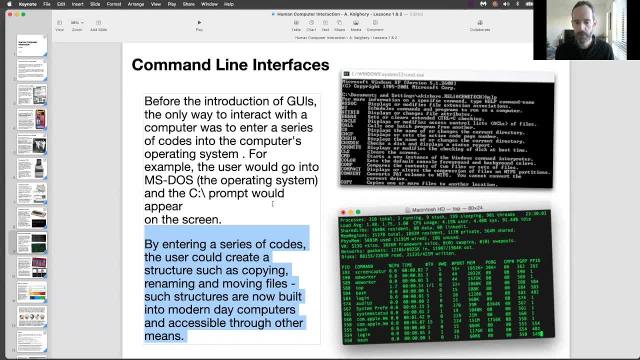 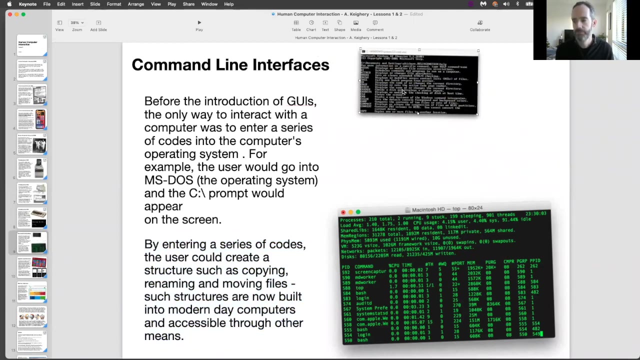 how would we do that on a modern day computer? so if I wanted to copy a file on my computer, how do I do that and say, say this image, all right. say I want to make a copy of this image, how do I do that? control C, yeah, and then paste: now I have. 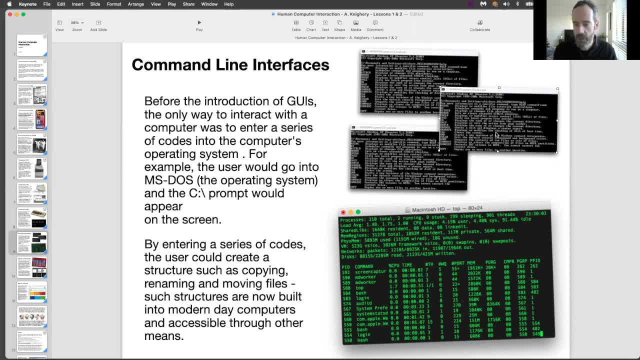 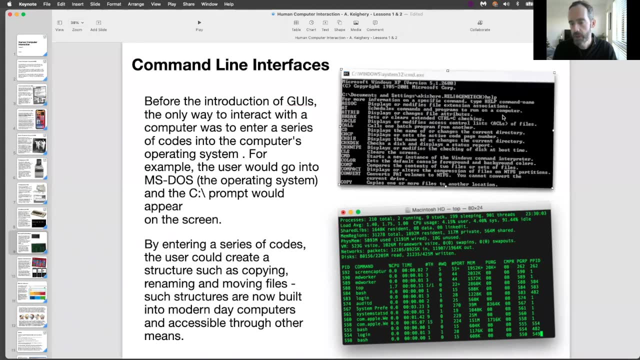 yeah, so it's that quick. so I'm on a Mac, so I'm hitting command C another way: click here, I go copy and then I go and paste. yeah, so so much more, uh, and then, if I want to change my mind, feedback: so much more convenient, right and much more user friendly doing it like that. 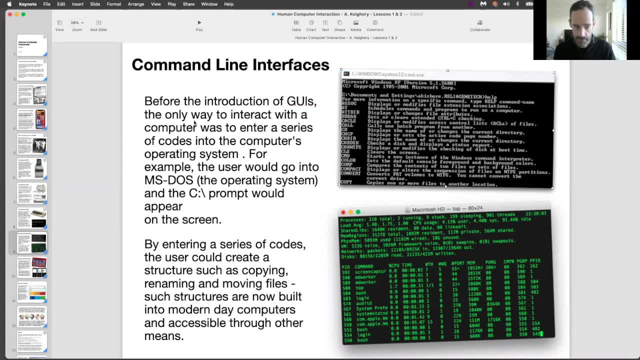 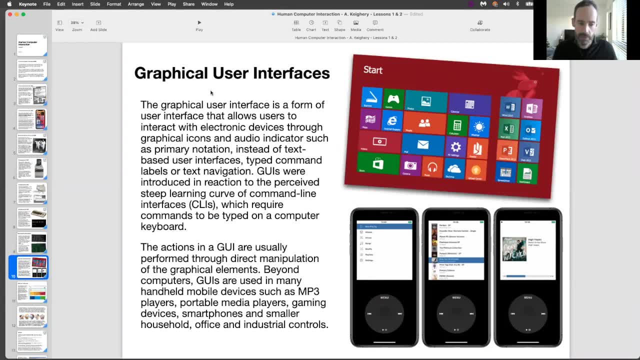 um, but typing in, I suppose, a load of codes using a command line interface, um. so graphical user interfaces, after command line interfaces, um, were around you. you had this emergence um of graphical user interfaces, you know, much more visually appealing to look at, um far more interactive, far more natural, far more learnable, right? so the graphic 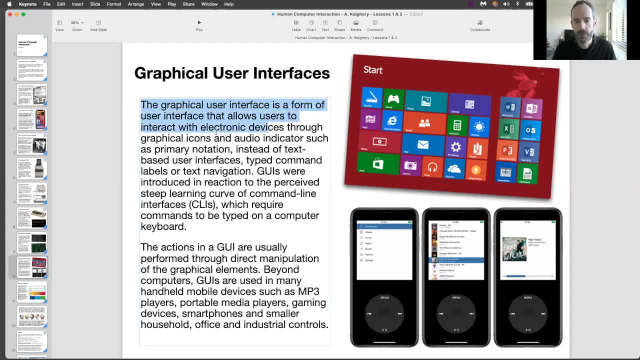 user interface is a form of user interface that allows users to interact with electronic devices through icons and audio indicators, and so, instead of typing text-based um commands and of having to navigate, you know a text-based screens- um guis- were introduced in a reaction to the perceived 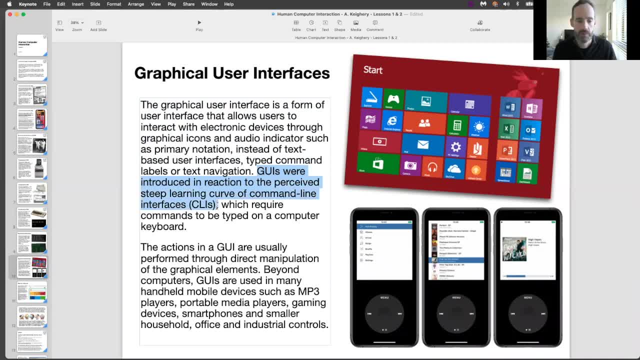 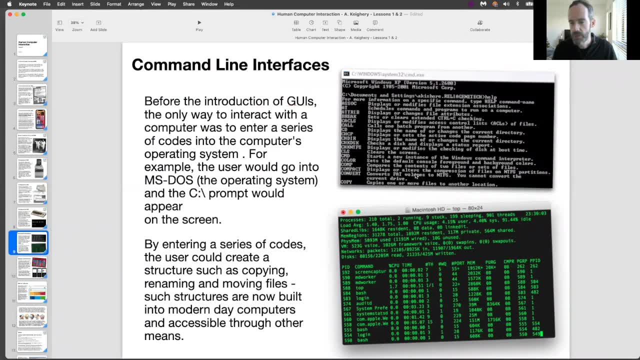 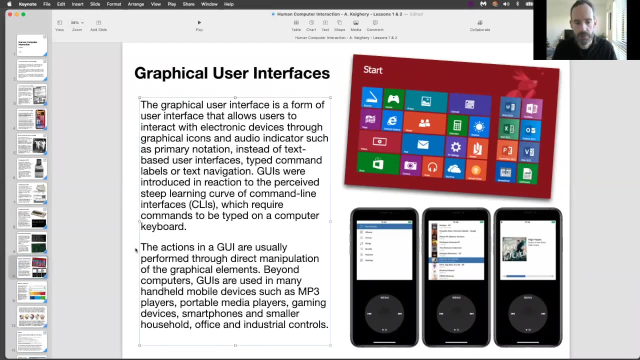 perceived steep learning curve in command line interfaces. so i suppose, look, they got invented because um these type of interfaces where you typed in the codes um for the computer to respond to were just very difficult to use and people struggled to use them. it was very specialized um knowledge. so the actions in a gui are usually performed um through direct manipulation of the. 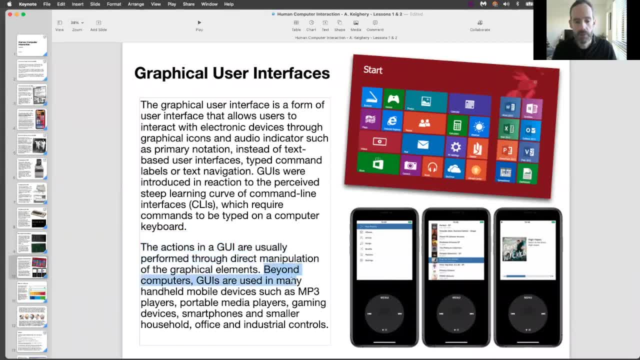 graphical elements and beyond computers, guis are used in many handheld mobile devices, such as mp3 players, portable media players, gaming devices, smartphones and and other households, um, items that are items that you might have in your phone. yeah, could anyone give me an example of a, a a device that has a user interface in your 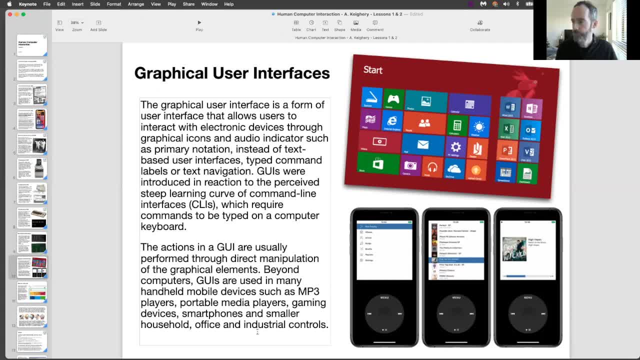 home. so say something from your kitchen. so what? what devices have user interfaces in your kitchen? any ideas? um, um, yep, um. smart fridge, yeah, because it would have a little screen. the oven- very good. the microwave, the dishwasher, the coffee machine- all these um different devices have, you know, interfaces, so they have some sort of a menu system and you need to go in and you 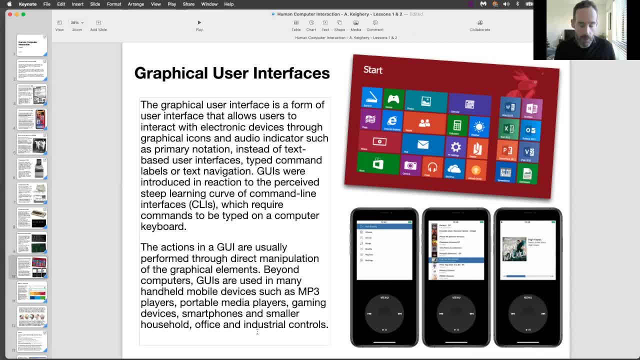 find what you're looking for. um, you know, a washing machine could have a screen or it could have a a series of dials and you twist the dials to get to the program that you you want. so remember, it's not just um computers and phones and that sort of stuff. so if you think of all the items um 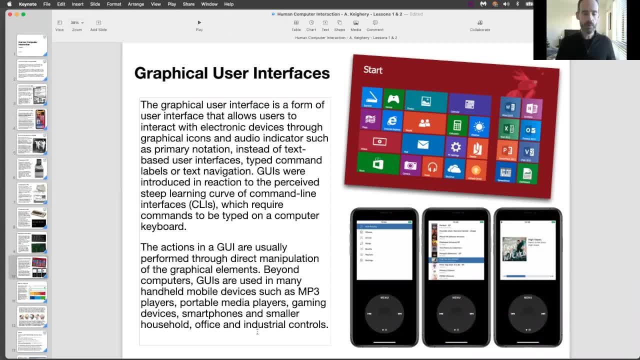 that that you use, you know even the, the way you interact with, with, with a car right, or the way that you know the train driver drives the, the, the train or the tram, like he has a set of controls in front of him and at some level people have sat down and they've said: right, put this here, put that. 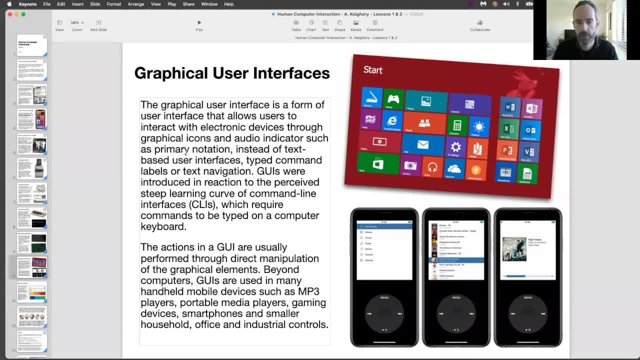 there, let's put that dial there, that sort of thing. so these are all interfaces of um different types. but generally when we're talking about graphical user interfaces, that's always um or tends to be within the realm of, you know, computer science and computers, laptops, phones, those type of things. so 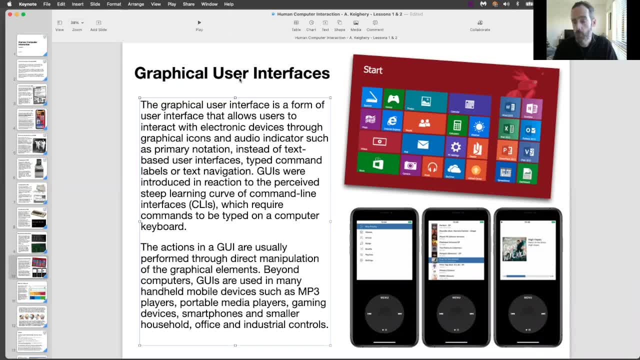 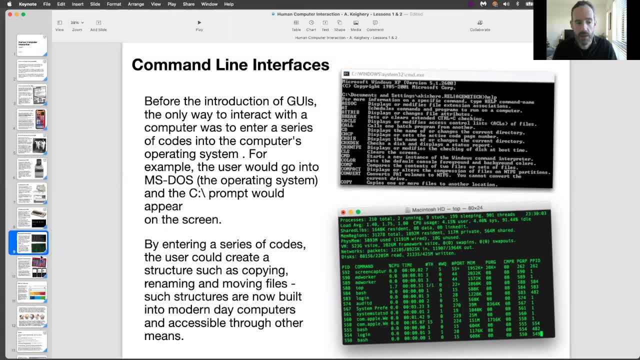 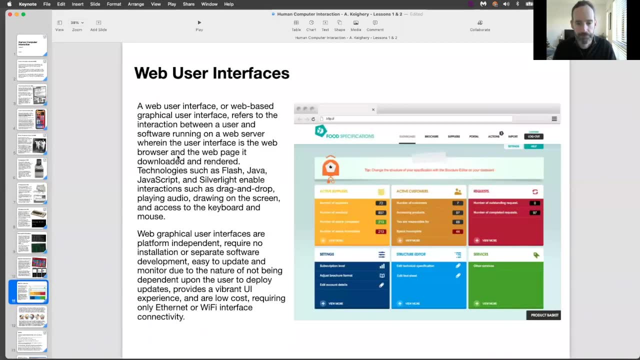 of devices, right? so the takeaway point is: look, graphic user interfaces. they replaced command line interfaces and they're meant to be more natural and more engaging, and now you see them on all different types of devices, right? so? another type of user interface that you're probably familiar with um web user interface. so this is: this is the type of interface that you see on. 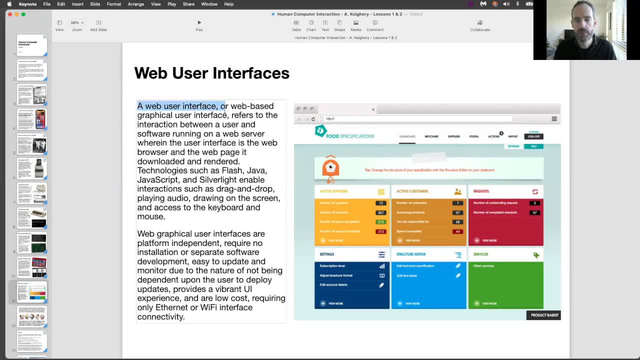 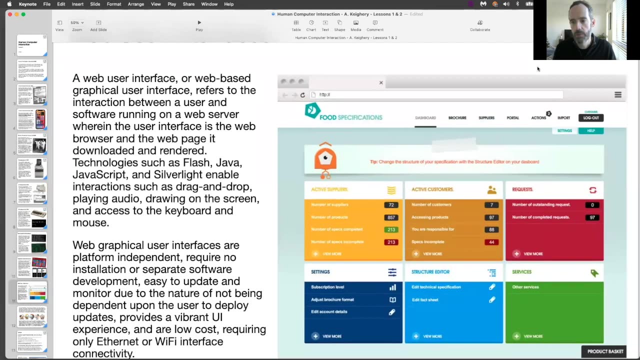 a web page, right so web user interface, um refers to the interaction between a user and software running on a web server right now. so, if we take this just- and i'll zoom in a little bit- if we take this as an example of a, you know, a typical web page, 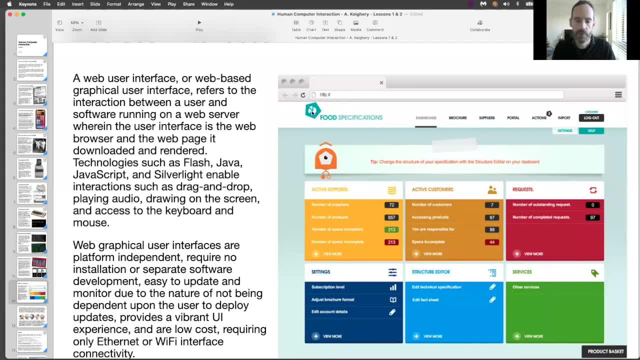 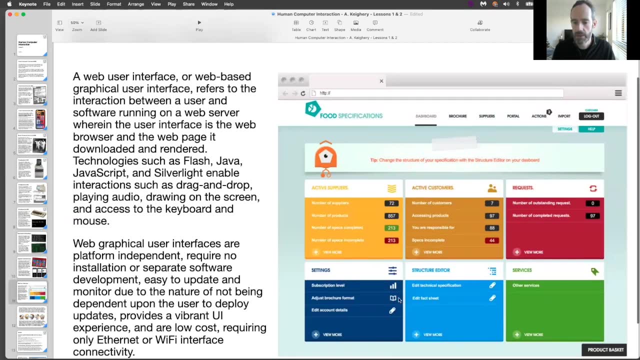 up the top here you have your address bar, you have the- you know the icon for the site, and then down here you have different sort of categories and they all seem to be grouped by color and that you've got yellow, red, blue and green and this type of stuff up the top. then you 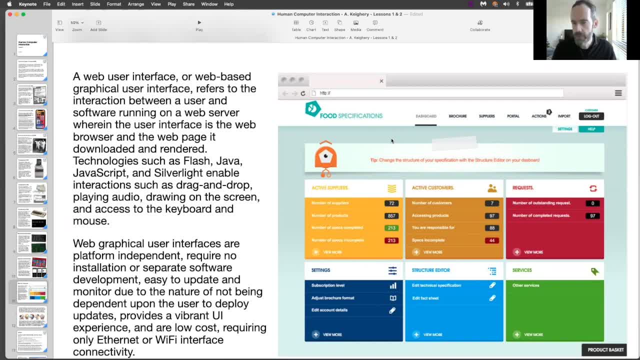 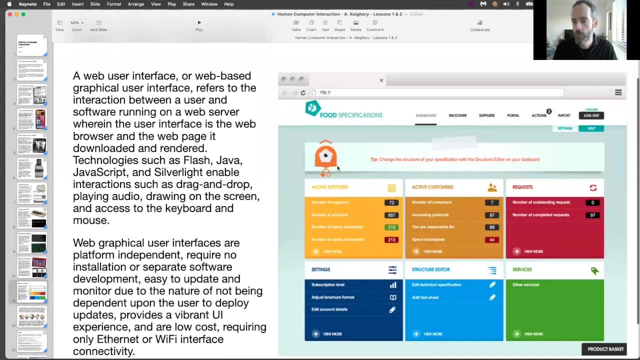 have a sort of a navigation system. so this is like the main navigation up here and this is the secondary nav where you get to go in to like a second um layer of information, and this is what is known as a web user interface, right, so web use, web graphical user interfaces, they're platform. 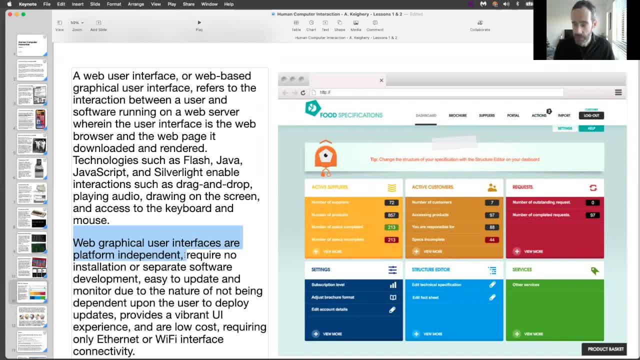 independent um and they don't require any installation. so i i don't install the website on my um machine, i just link to it or i link to the web server using my browser, so using safari or firefox or internet explorer or one of these um applications, um the any, any. they're easy to update. so if the web developer or the company wanted to make a 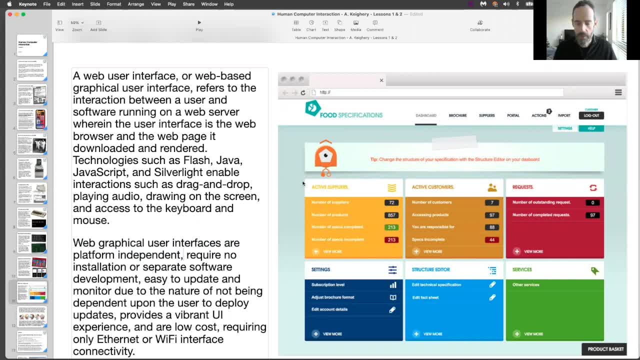 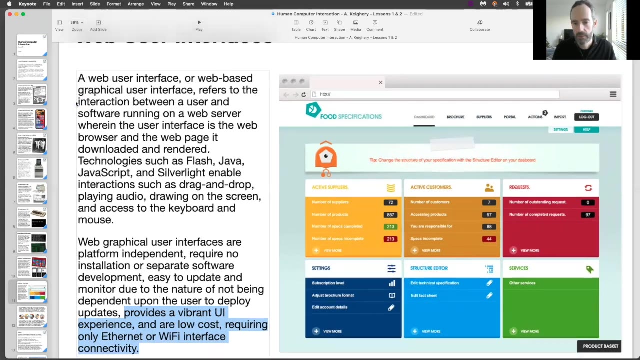 change on this. the next time i visit the, the site, um, you know, i can see those changes and that sort away. so, um, yeah, so they provide a vibrant user interface experience and a low cost um for me as the user to to access, right? so that's just another example of um, an interface, and we call them. 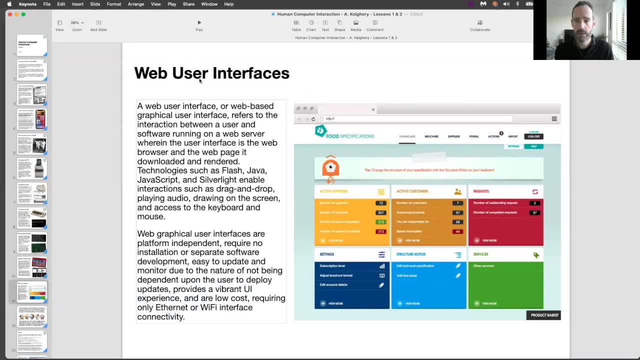 web user interfaces. so so, if you think of any um any website that you've visited recently, when you go in and you interact with the menu systems on the side, and you go and you click around the side, you'll you'll see how the information is grouped and and how it's structured. 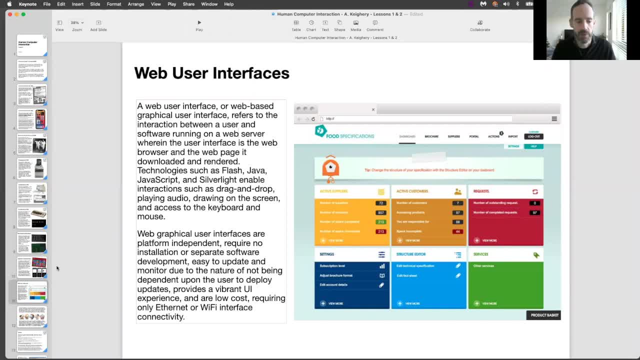 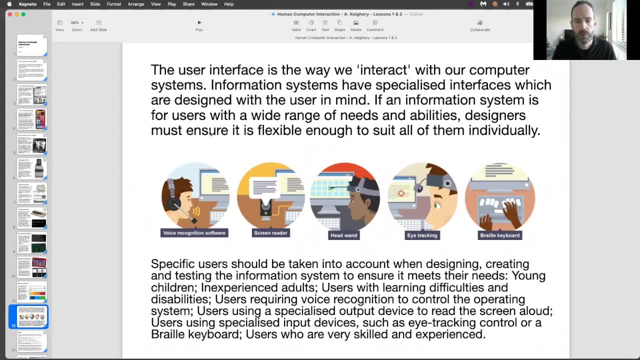 and what your web browser is doing, but again an example of another type of interfaces. so, um, we'll look at maybe more specialized interfaces for a couple of minutes. so the user interface is the way we interact with our computer systems, and information systems have specialized interfaces which are designed with the user in mind. 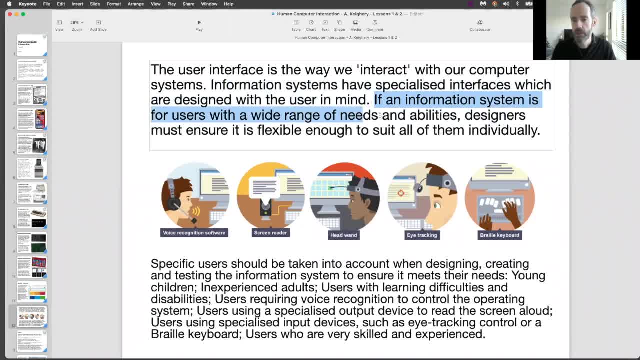 so if an information system is for users with a wide-ranging of needs and abilities, designers must ensure it's flexible enough to suit them all individually, right? so what you're talking about here is maybe a user cannot use a computer or a phone or the interface in a traditional sense, so they might struggle to use the mouse or the you know there. 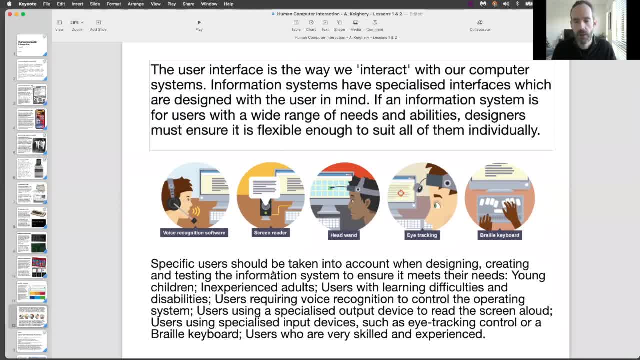 could be mobility issues, site issues, all these different things. so then there is like an onus on us as developers to try and develop interfaces that are, as you know, inclusive as possible. so you have things like voice recognition software and screen reading software and you- you have seen, 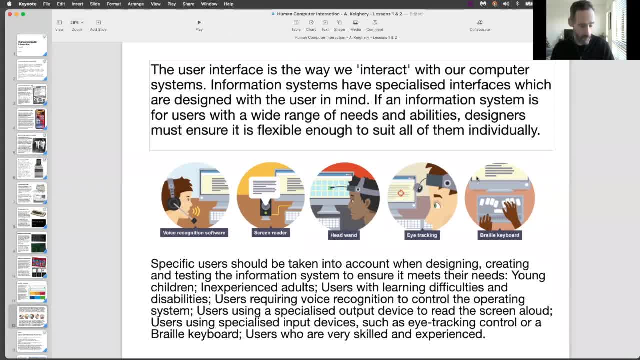 head wands, eye tracking and we have keyboard for people who, you know, struggle with their sight. those type of things and specific users should be taken into account when designing, creating and testing information systems to ensure that it meets their needs. so you're talking about all different types of. 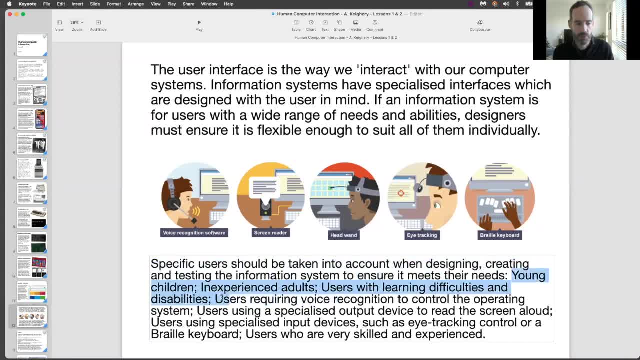 users- really, you're talking about young children, right- inexperienced adults, users with learning difficulties and disabilities, and users that might require voice recognition to control the operating system, and users using a specialized output device to read the screen loud- well, all those kind of things. and what that does is it makes the computer system more inclusive and more useful. 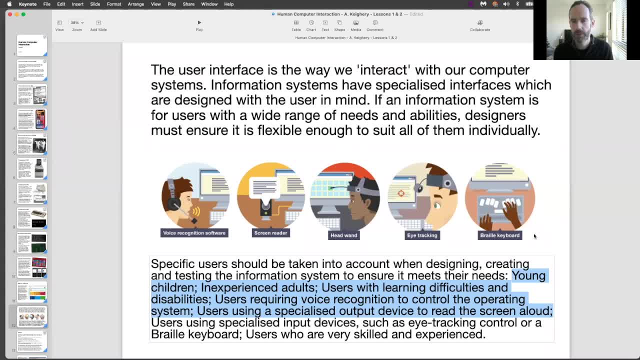 right, but you know that a lot of these things would apply to me as well. i know my phone has a digital function so that when i'm driving if i receive a text message, then the phone will actually read the text message to me. so i don't need to look down at my phone. and when i'm driving 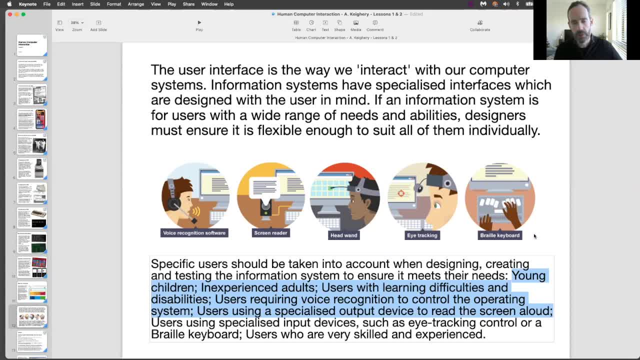 and the more adaptable these computer systems are on these devices are generally, the more useful they are to- um, you know, to a lot more, a lot more people, right so i suppose, look as interface designers. it's important to bear in mind these factors. um, when we're looking at, you know, let's say there's a firmware at work, let's look at the performance of a device in the future to see which one of them will succeed. 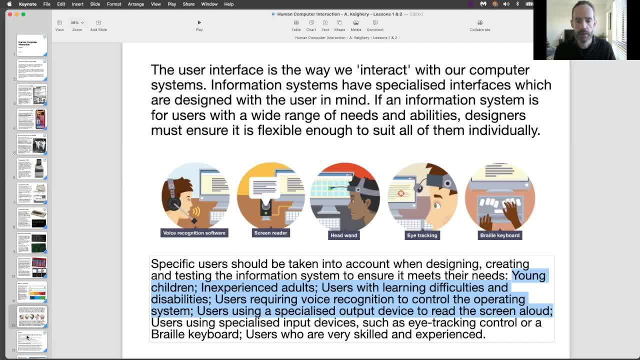 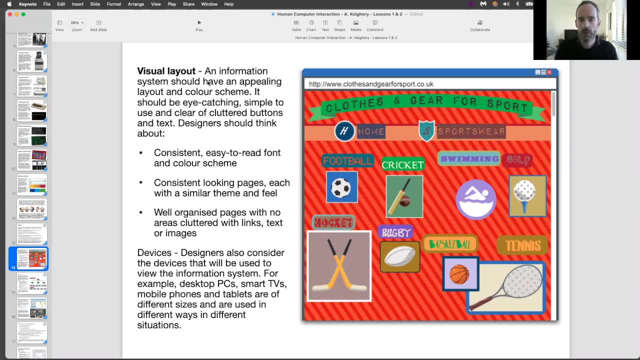 we are designing and constructing interfaces. Okay, so the visual layout, right. so now, if you just very quickly compare this layout, so this is a web page, so how do you find this to use? So, if you just look at that very quickly, what does it strike you as? 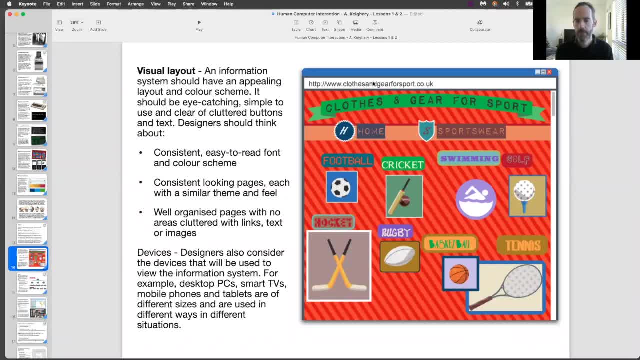 So does it? does it appear easy to use? Yeah, it's really bright, so the colours are a little bit off, almost right, so can too many colours. yeah, the fonts- look at all the fonts are different, so there's no uniformity. Now, if 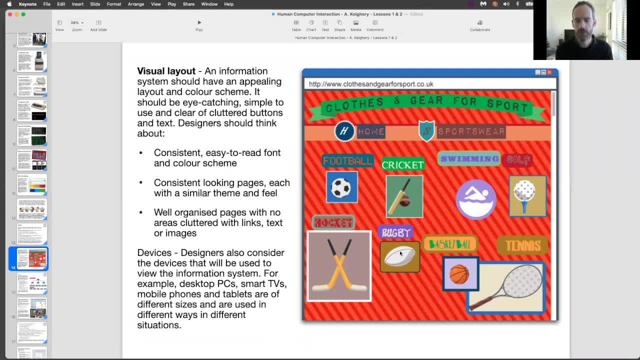 you wanted to find something on that. is it difficult to find what you're looking for? Yeah, so it's just, it's hard to, yeah, it's hard to find what you're looking for because you've got all these separate things, you know, grabbing for your attention. So if we, if we compare that, 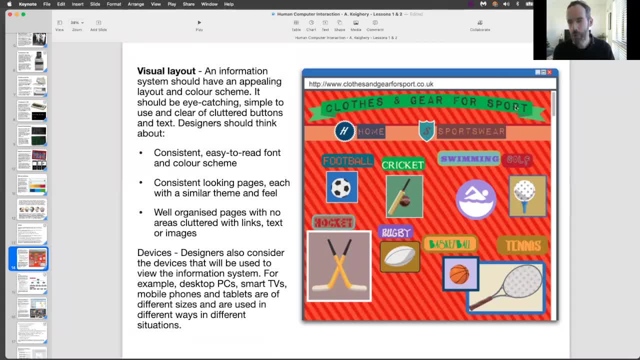 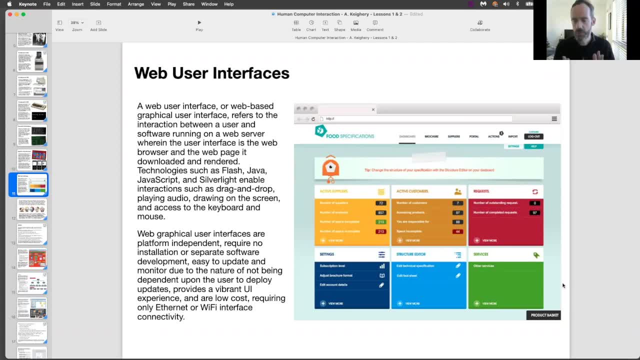 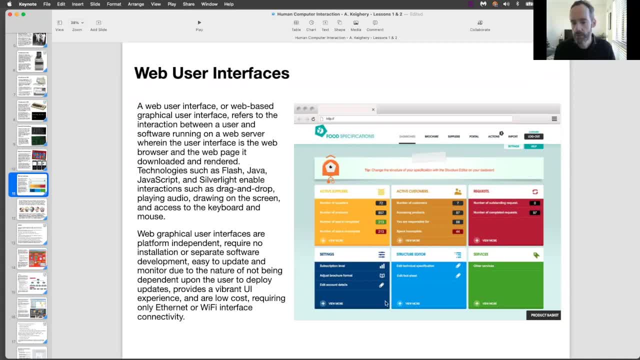 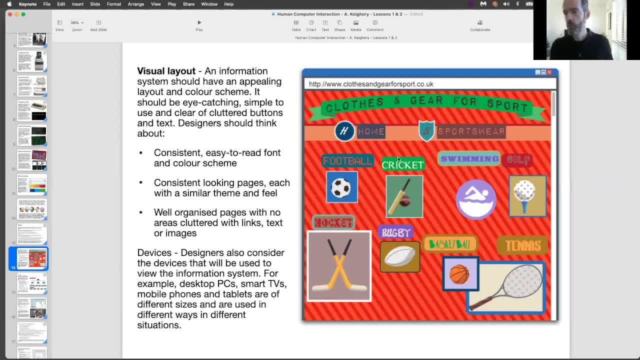 there's our bad example as well, and you, honestly, you don't know if that's a web page. you don't know where to click or what to, or what to do with it or anything. so this is in terms of a 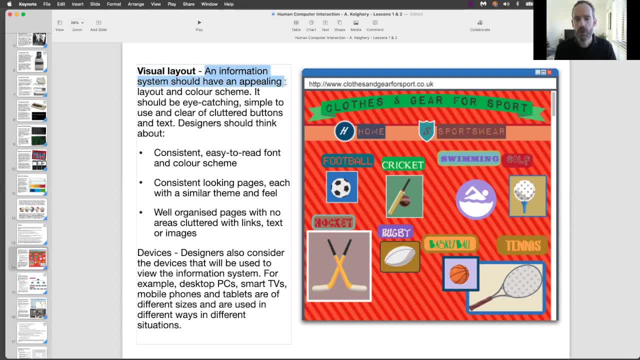 visual layout. so the information system should have an appealing layout and colour scheme right, and it should be eye-catching, simple to use and clear of cluttered buttons and text. so you're looking for things like consistency, easy to read fonts. 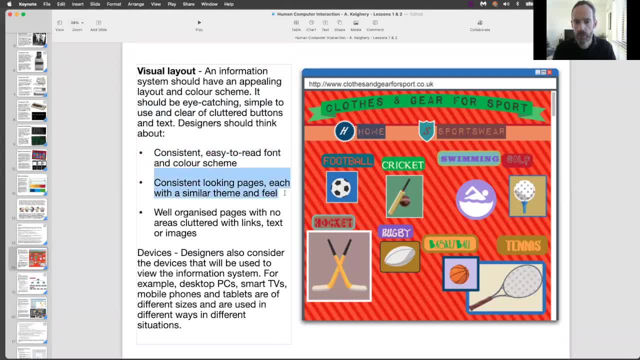 and colour scheme, a consistent look across pages, well-organised pages with no areas and links and text and everything is wrong about this. so all the images- they're not aligned, the the it's just yeah, and even then the background as well really catches your eye right. 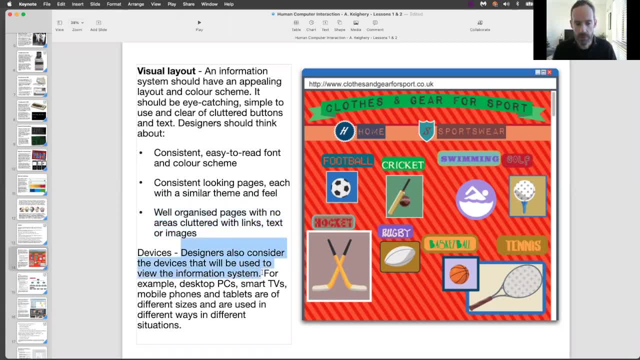 designers also consider the devices that will be used to view the information system. so you have to think as well where is my information system or where is my interface going to appear? and because you know it's a very different thing looking at a phone. 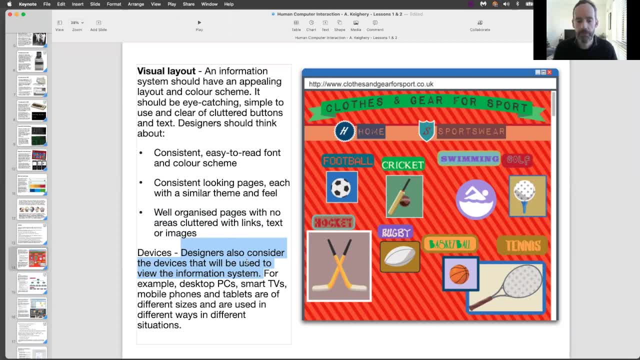 than it is from looking at, you know, a big smart TV or something like that. so when you're you're, you're thinking about trying to design an interface. sometimes you have a you know, a particular device in mind and you know as well. 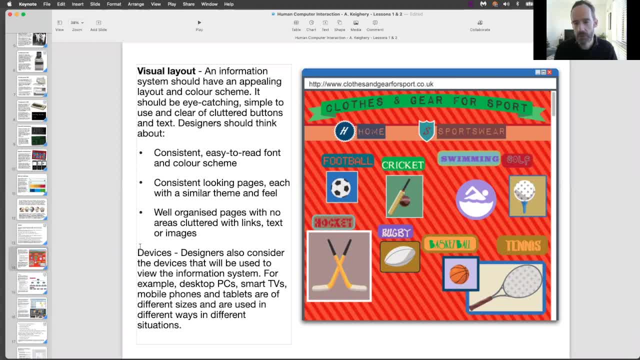 how much screen space that you're actually going to be working with, right? so this? just take this as an example of a very bad design. bad because it's not consistent. everything's cluttered, the images, yeah, just every. everything's wrong with this. so the visual layout of the page is 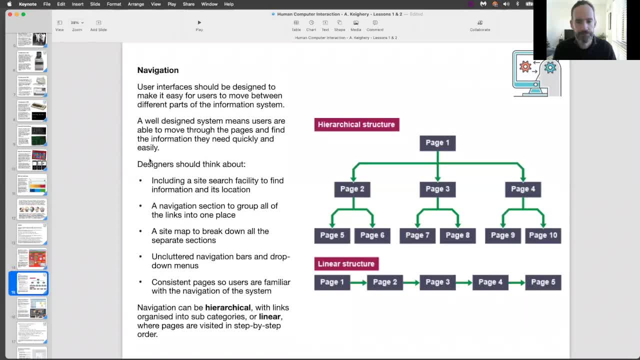 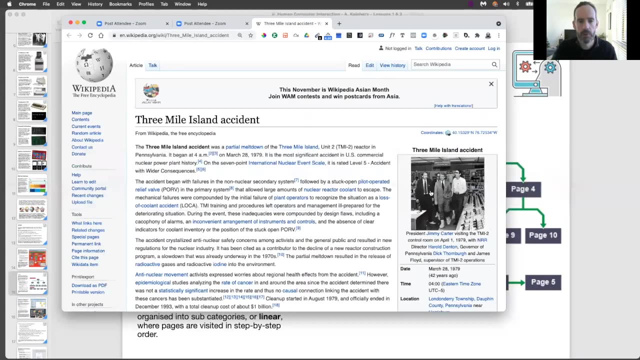 is completely. it's just poorly put together. and this brings us on to to navigation. so your navigation then on your site is how the users move around the site. so we're giving it a site with. I'll give you an example of, say, navigation. 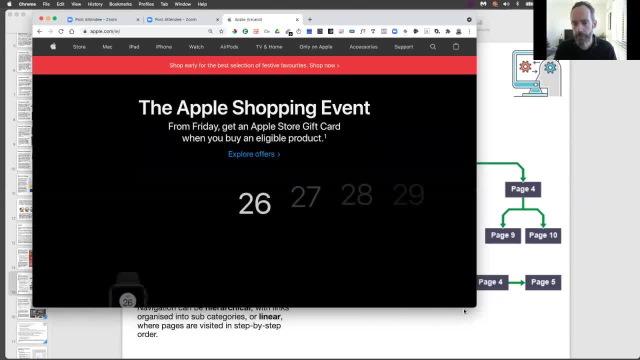 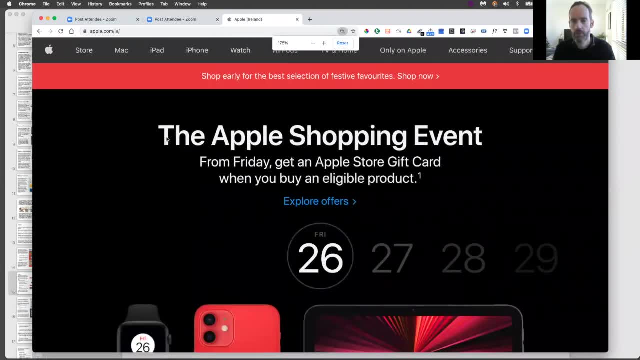 and so we go to a site like Apple. it's very well thought out and well designed, so. so where's the navigation menu here? so here's my, my main navigation, right, and then as I go down the page, 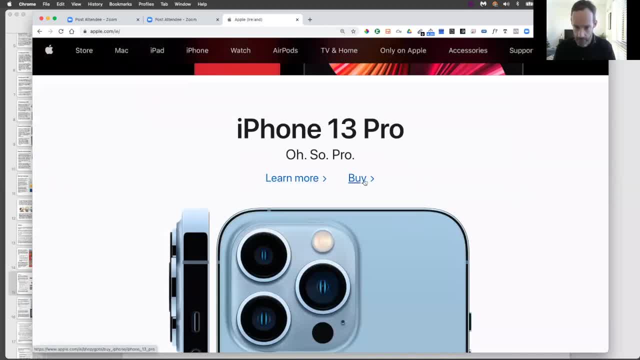 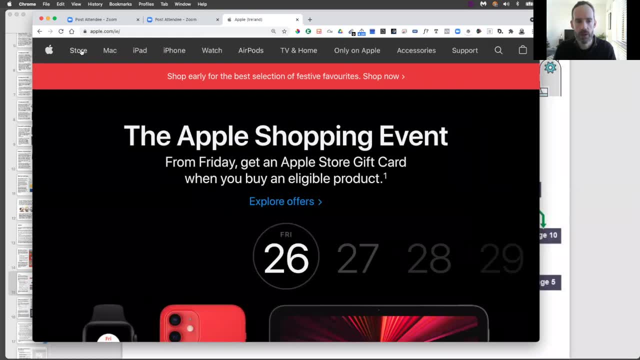 I get options to go into. you know, other areas of the site, but you can see that this banner along the top doesn't really change. so these, these are the main categories of the products that Apple- that Apple, you know- offer, offer me. 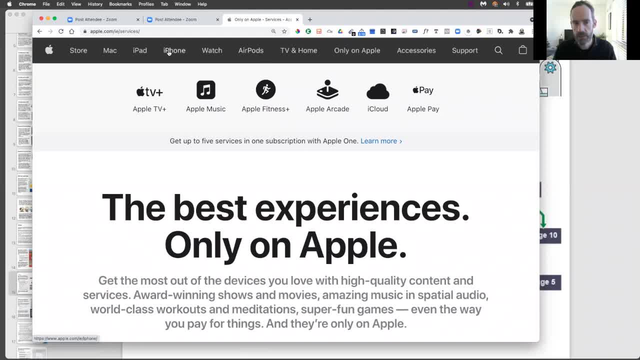 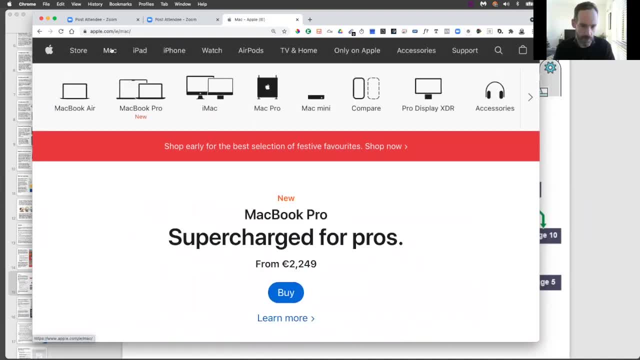 so, and each one of them, when you click into it, you'll get sort of a like, almost like a sub category where it pops up. so if I click on Mac, it'll show me all the computers I can buy, you know. but again, it's given me text to work with, it's given me a graphic. 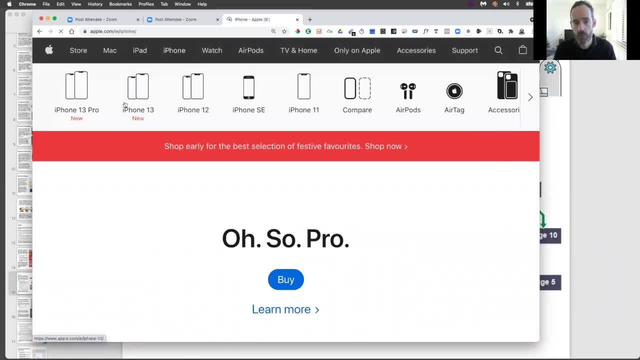 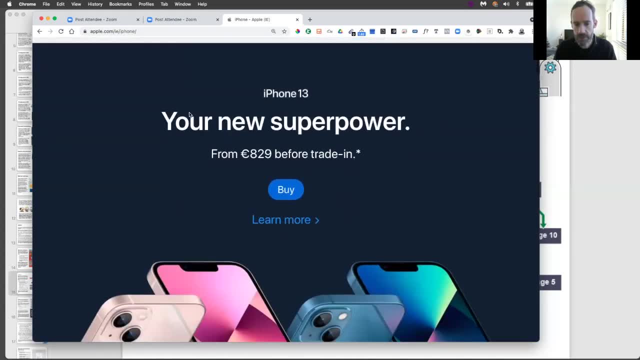 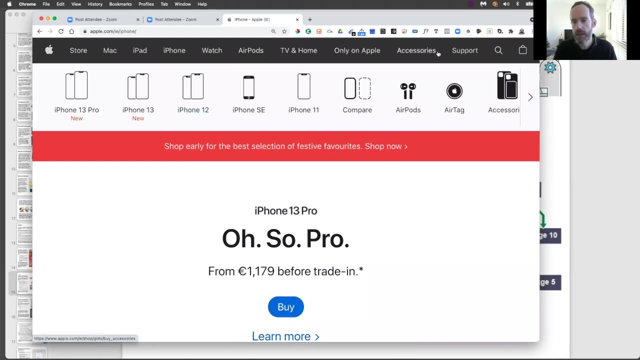 look at. if i click on the phone, it'll give me a list of all the phones that i can buy, so it's generally well put together and very consistent. color schemes, nice pictures, this type of stuff. but this main area across the page is known as your, your main navigation. right, you can actually 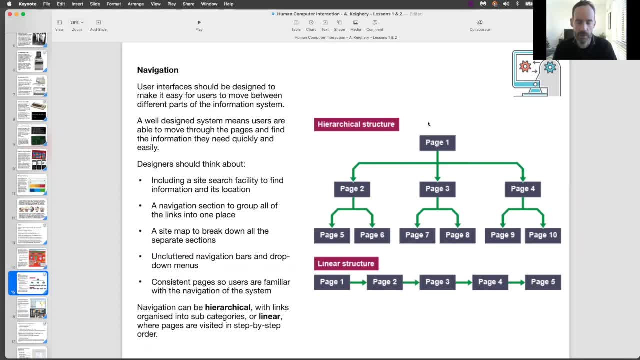 see that this, the site, follows a kind of a hierarchy, or you can. you know, you can get around it and using certain means. so this is like your home page and then after your home page, you have options to go into secondary pages and then you have another layer and most um. 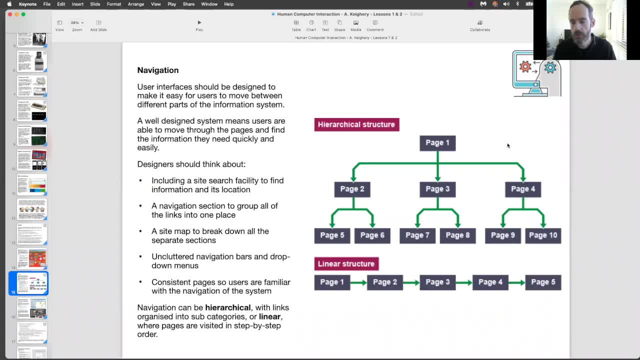 websites are put together using this hierarchical sort of structure. right, and with some menu systems you see a different type of structure. you see a linear structure. so this is more like the pages in a book, where you have to go one, two, three, four, five and then you're back to the start again. so you see a lot of menus on tv systems like that, where you have 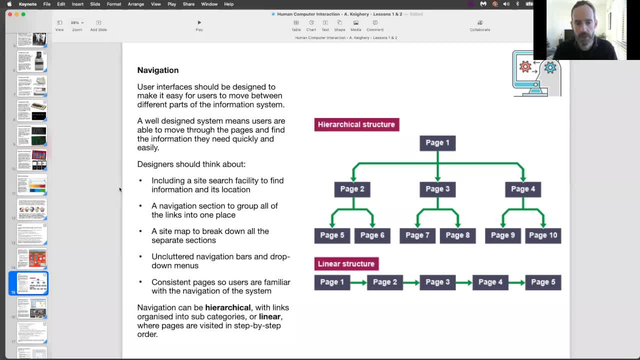 to scroll through um different different pages and what have you so again look? the point of making is that the navigation of the site and is important and generally, this hierarchical structure is one of the ways that um, that designers um put the site together, and it's what we're used to looking to as well. 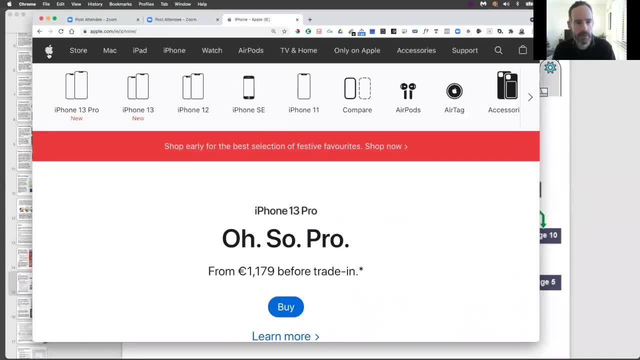 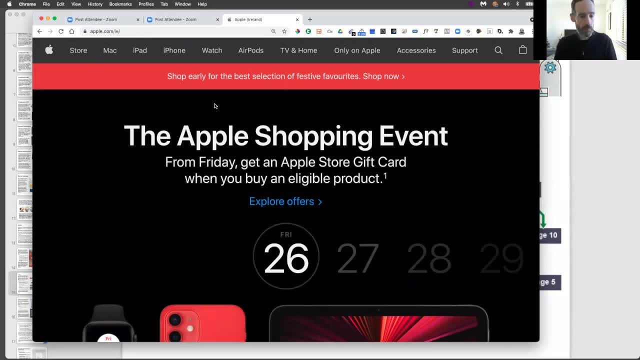 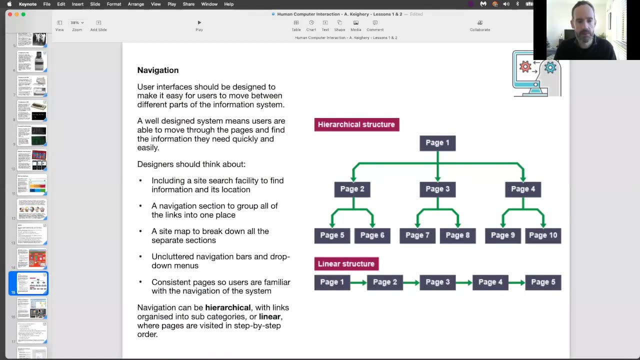 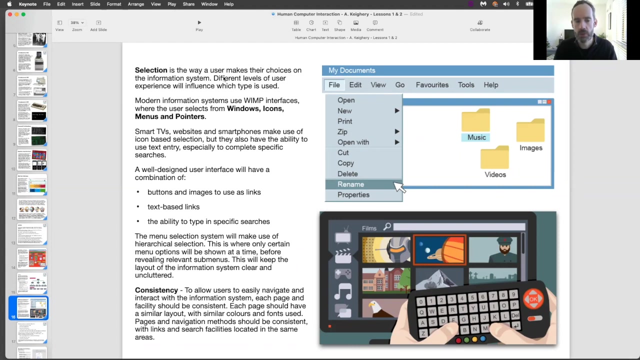 you know, if you go to any website, you'll see these examples of um. you know, a landing page, secondary pages and sub areas on pages, all that kind of um stuff, so that learnability is a factor as well. um, so selection is the way a user makes their choice. 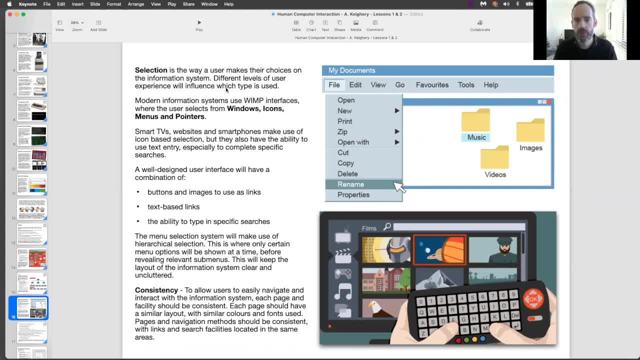 is on the information system and different levels of user experience will influence which type is used. so modern um computer systems use wimp interfaces where the users have windows icons, menus and pointers. so if i'm using this um slide software keynote that comes with mac. so if i click here, these are all the different commands, right? so i go into the top and then i go. 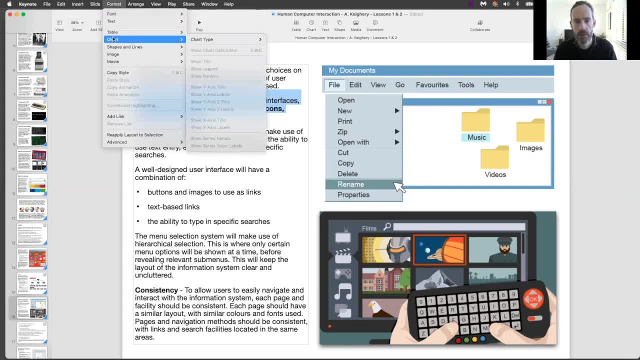 down, and then you see the secondary kind of commands that are available to me. you see those up here, right? so this, this is a wimp system. so remember windows icons. so the icons are just, you know, graphical representations, so it's a beast type of things: folders and windows, and 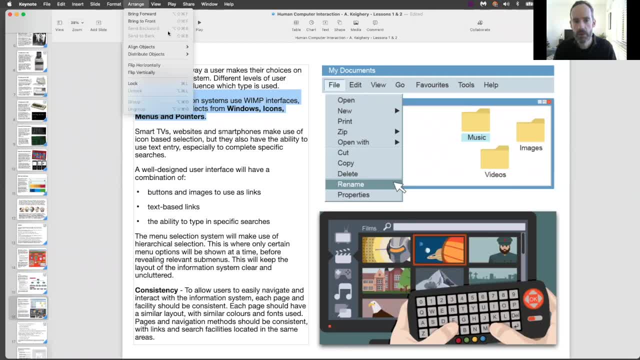 menus that you can click on and then they appear, so that that doesn't appear until i click. and then my pointer, which is, which is my max? so smart tv's, websites and smartphones make use of icon based selection and but sometimes they also have the ability to use text entry, right, so you? 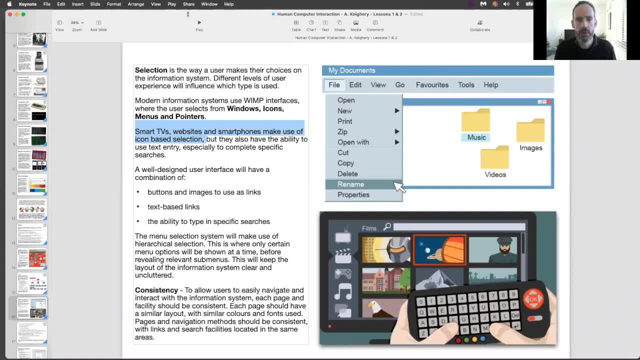 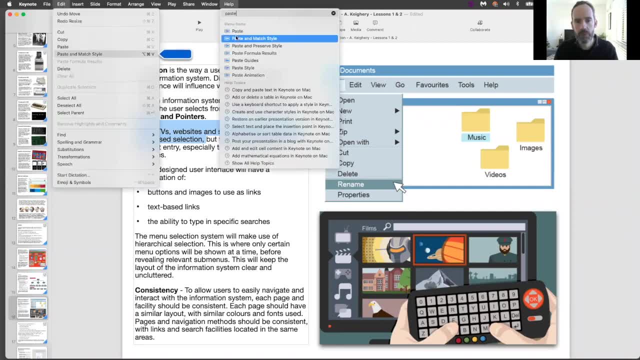 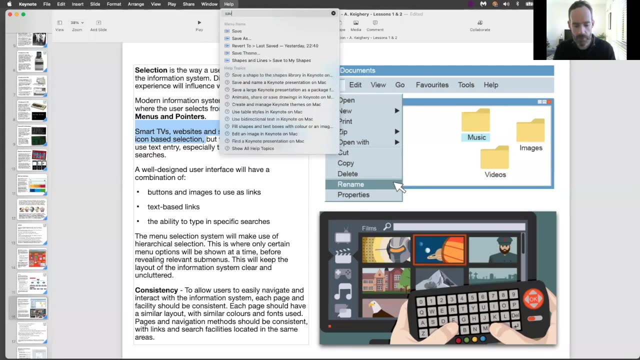 might have the, the um option. so if i go in here, see, so it even shows me where. so if i'm looking for, uh, a command, so something obvious like save, so i type in my search, so it's like a search engine for the app and it actually takes me to. so it shows me which menu, the particular um, the 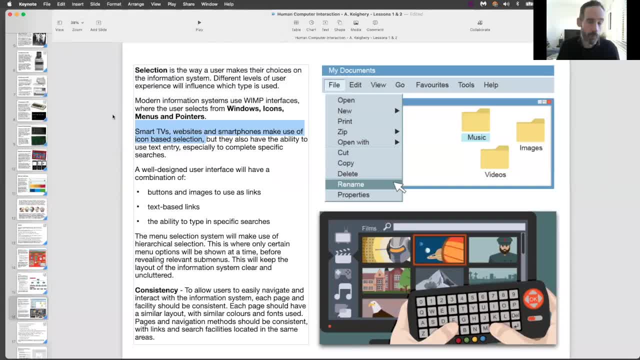 particular thing is in, so there can be different ways to find things on different websites. so a well-designed user interface will have a combination of buttons and images to use, as well as links. it'll have text-based links, um, and the ability to type in specific searches, right, so that ability to search as well is kind of like a catch-all. it can be. 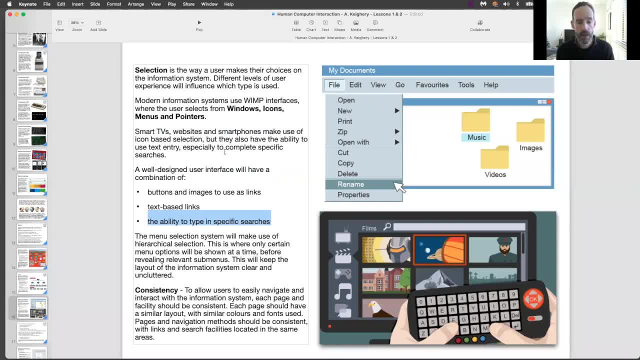 very helpful for users as well, and you see it on a lot of um interfaces and a lot of websites. so, say, using this example, this looks like some sort of a console or a smart tv and you can move around the interface. you can use the arrow, use the arrows, you go up down, left, right, a little bit like the way you scroll around on Netflix or 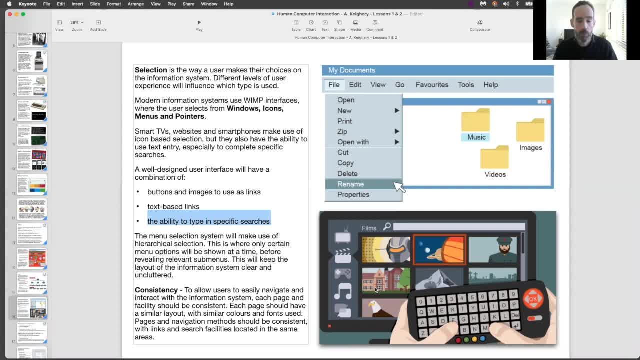 something like that, and then you make your selection, which you can also pull up a keyboard and you can actually type in a search and it will give you results back as well. right, and the key to all that, I suppose, is consistency and to allow users to easily navigate and interact with the 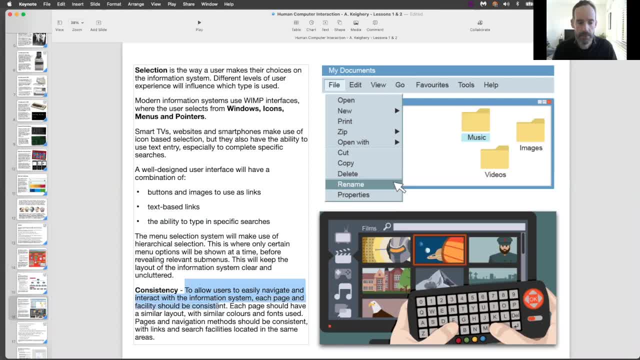 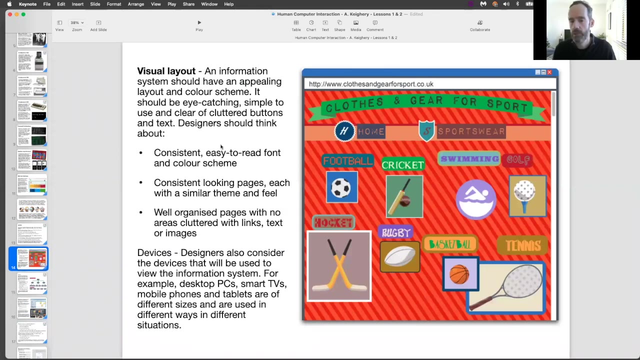 information system, each page and facility should be consistent and each page should have a similar layout, with similar colors and fonts used, and pages and navigation methods should be consistent with link and search facilities located in the same areas. right? so just think of our bad example again, right? everything is jumbled, everything is. 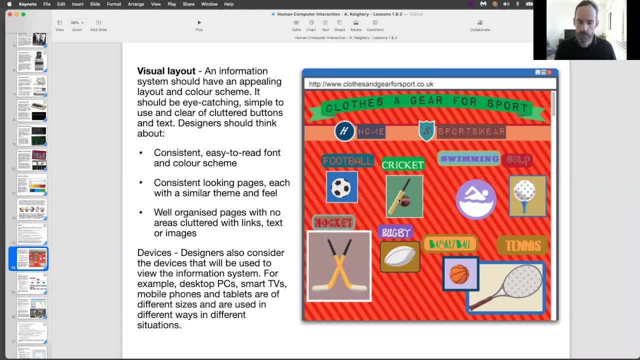 just fields off the colors, the icons, the size, the fonts, all the all, all the components of the page that we, we, we expect are, I suppose, you know, not as they should be. think of a good example, then, something like you know one of the Apple website, the Netflix app, these type of things, where